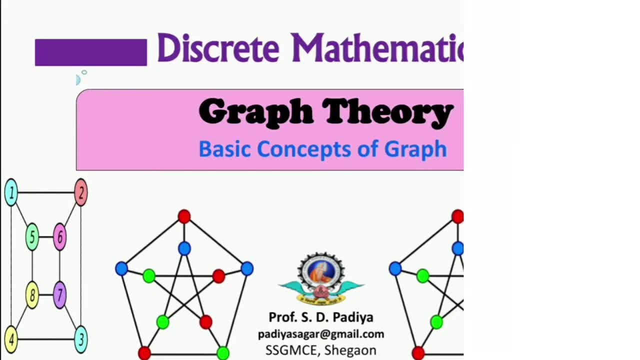 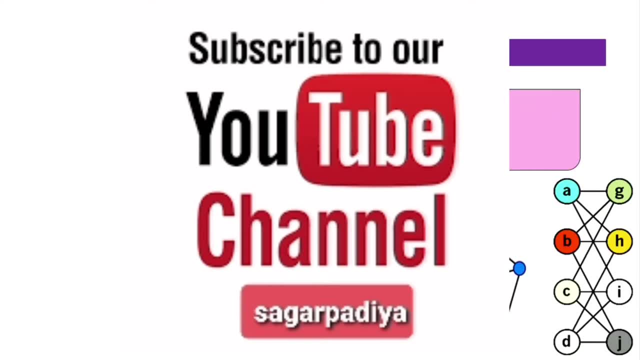 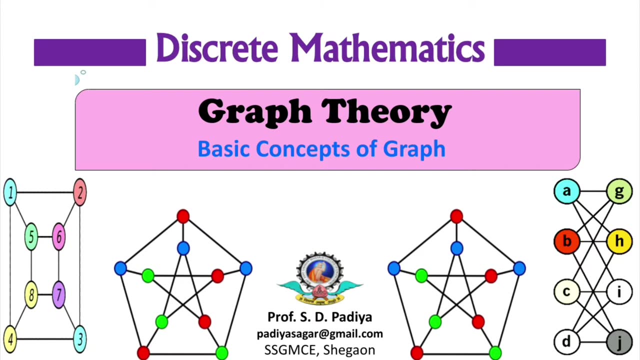 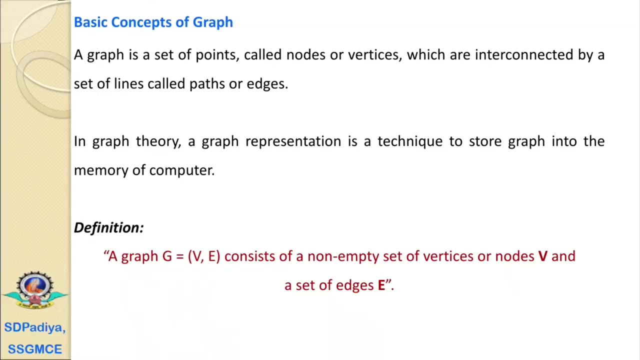 Hello guys, in this video we will learn about basic concepts of graph theory in the discrete mathematics. I am Professor HD Padia from SHGMC, Shegaon. A graph is a set of points called the nodes or vertices, which are interconnected by a. 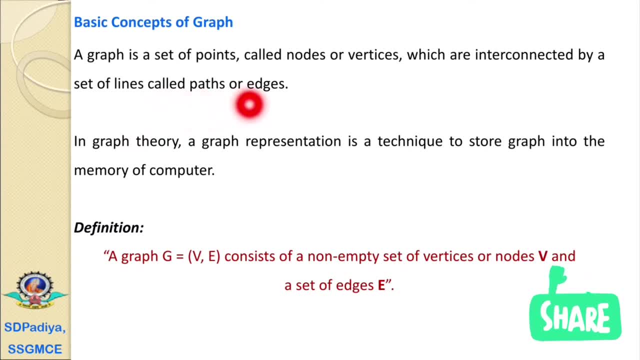 set of lines called the paths or edges In a graph theory. a graph representation is a technique to store the graph into the memory of computer. The definition for the graph theory is a graph which is denoted as a capital G, which is a ordered pair of V- E, where the V it is a non-empty set of vertices or nodes or vertices. 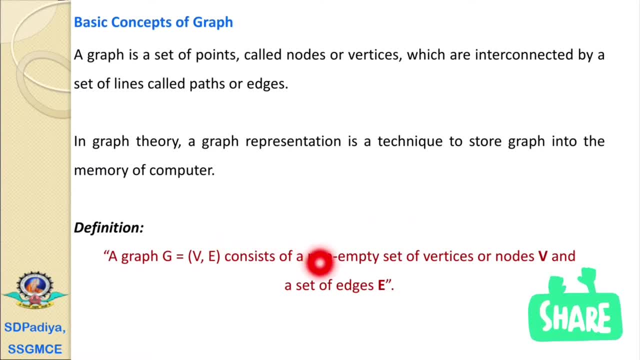 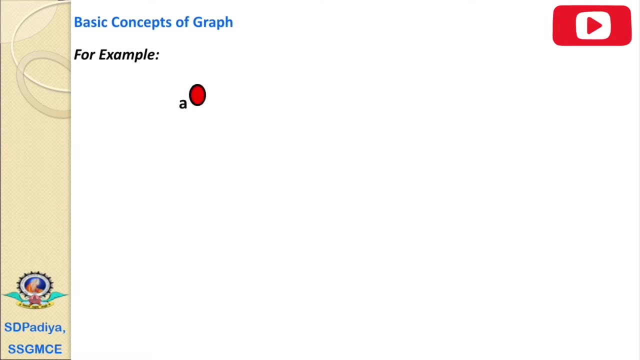 or nodes, and the capital E. it is a set of edges. That is, a set of vertices and a set of edges. it is called a graph. We will have the one example here. Suppose we have the four vertices A, B, C, D. Now there is an edge between the nodes A and B, between the 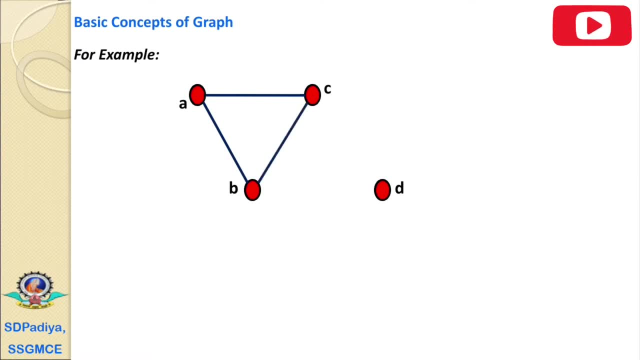 C, the edges between the B and C, and there is edge between C and D. Now here the A, B or it is considered as the BA. The edge is considered as A, C or CA. The edge is considered as BC or CB and similarly, for the last, the edge is considered as the CD. 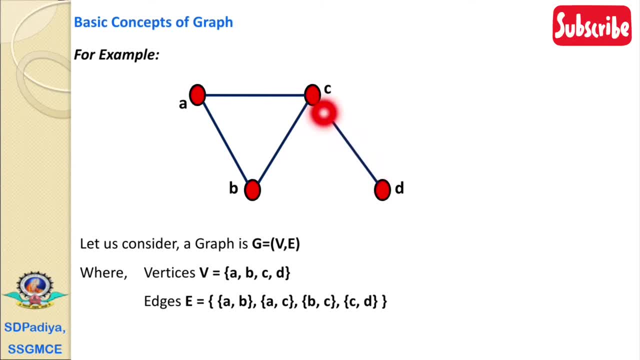 or D, D, C, because there is no direction is defined Now. this graph is denoted as an ordered pair of V, E, where the V it is a set of four vertices: A, B, C, D and the capital E it is a set of four edges. 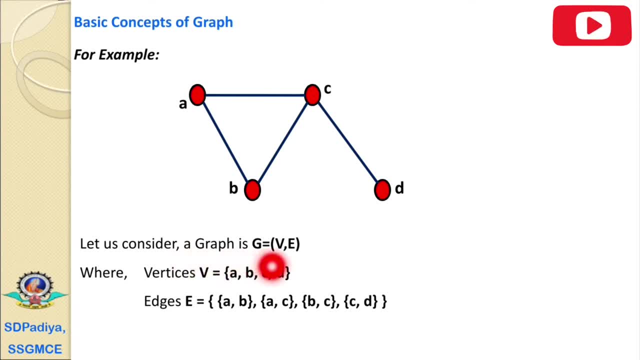 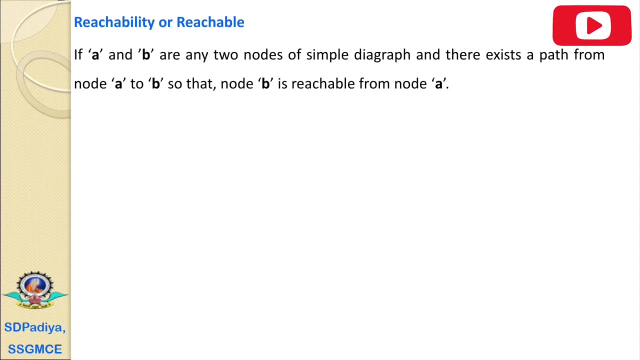 the A, B, A, C, B C and the C D. Now these four edges are undirected. therefore we have defined in the unordered pairs, that is, by the curly braces. The next concept is the reachability, or reachable. If we have any two nodes, then it is not compulsory that both nodes are reachable. 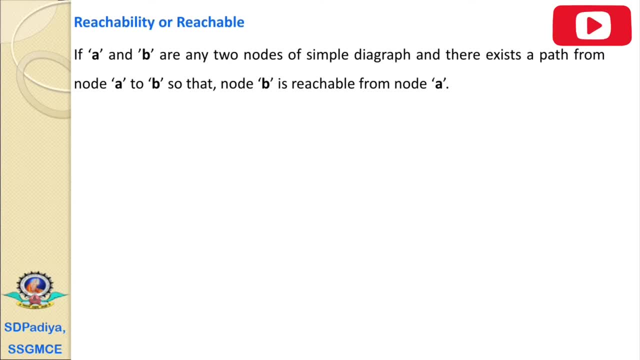 from one node to the other. So if we have any two nodes then it is not compulsory that both nodes are reachable from each other. It is depend on the given direction. If A and B are any two nodes of a simple digraph, the digraph means it is a directed graph and there exist a path from. 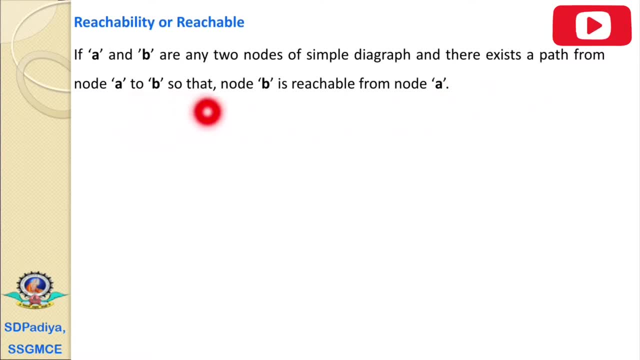 the node A to B so that the node B is reachable from node A. The length of the path from the node A to B is not compulsory. So if we have any two nodes then it is not compulsory that both nodes are reachable from one node to the other. Now the next concept is the flow of distance. 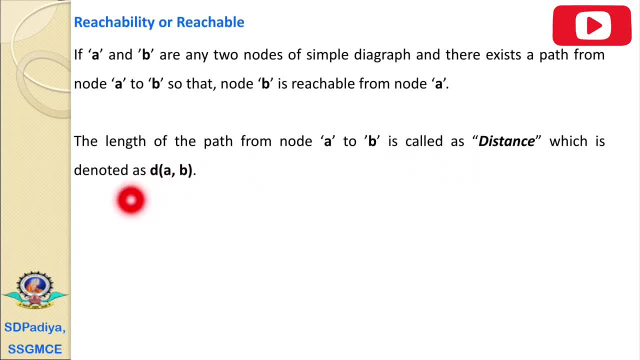 So in the example here of A to B it is called a distance and it is denoted as the D of A- B. that is the distance between the node A and B. We have the example here Now. in this example, 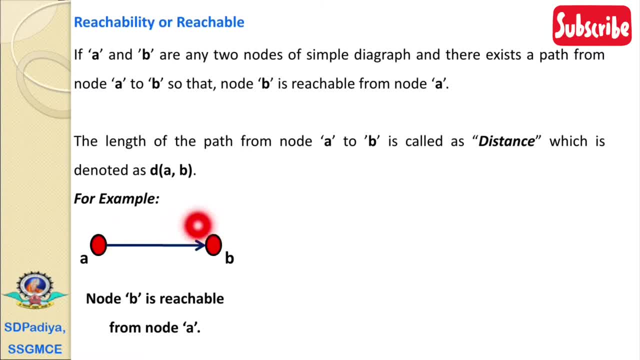 the two nodes A and B, and the path is from A to B. there is a direction that not mean it is from B to A. Therefore here the node B is reachable from node A. In the second example now, the node A is reachable from node B. Both are different. 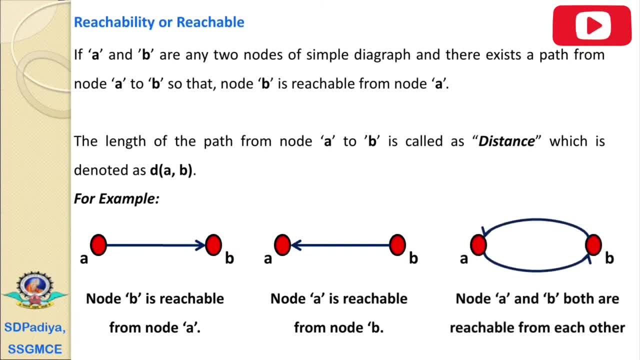 And there may be a pair of any two nodes in which both nodes are reachable from each other. If we look to the third example here, node A is reachable from node B and the node B is also reachable from node A. Therefore we have written that node A and B both are. 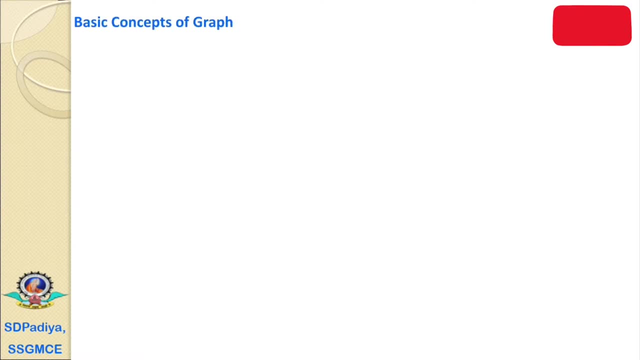 reachable from each other. Now the next is the degree of a vertex or node, The. every node has a degree. Your degree value may be 0,, 1,, 2,, 3,, 4,, 5,, 6,, 7,, 8,, 9,, 10,, 11,, 12,, 13,, 14,, 15,, 16,, 17,, 18,. 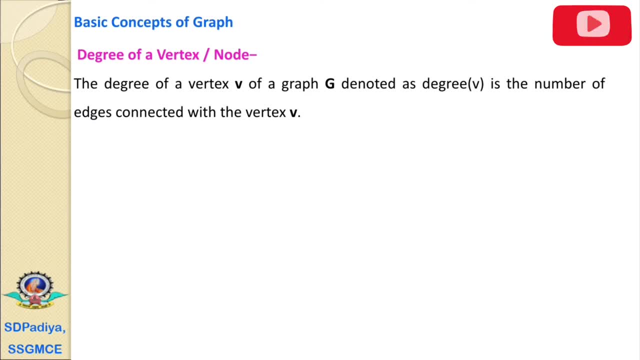 19,, 20,, 21,, 22,, 23 up to the n. The degree of a vertex V of a graph G, denoted as a degree in bracket V, that is, degree of vertex V is the number of edges connected with the vertex V. 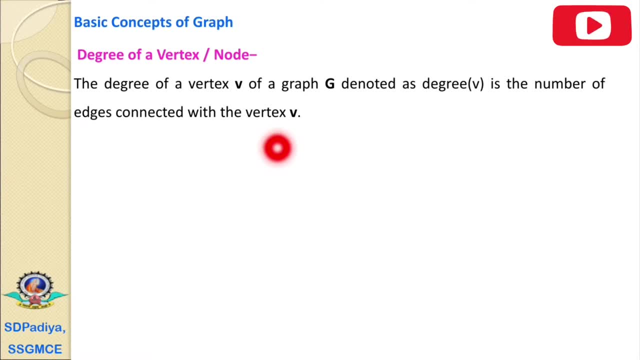 To the any node how many number of edges are connected. it is called a degree of vertex. Now we have seen the two types of vertex. So now we have seen the two types of vertex. Directed edges. The edge may be incoming towards the node or edge may be outgoing from the node. 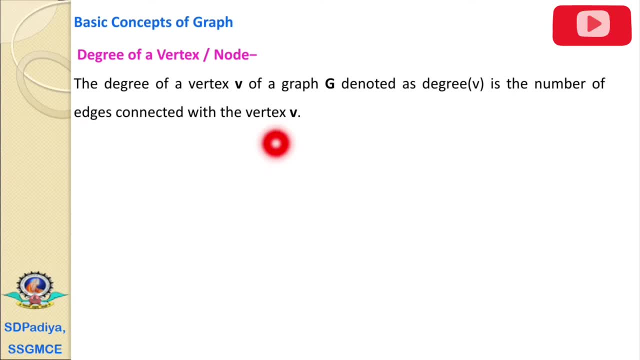 Based on this incoming and outgoing edges. we have two types of degrees. The first is n-degree of a vertex V, denoted as n-degree in bracket V. that is n-degree of vertex V. It is a number of edges coming into a vertex. 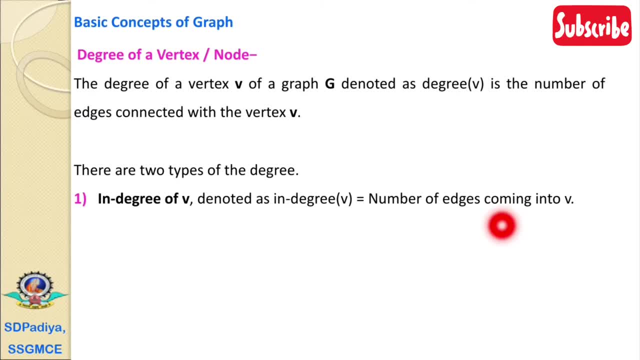 V, that is number of incoming edges. that is called in degree. the second is out degree of a vertex V. denoted as out degree of V, it is a number of edges outgoing from the vertex V. now in a graph there may be any node which has only the out degrees and zero in degree. then a node V is called source if it has. 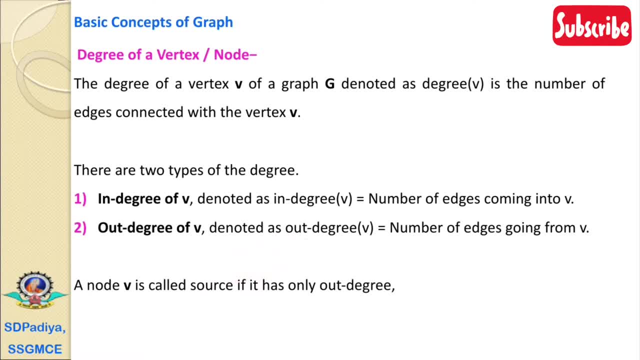 only out degree. it is example for source node. or in a graph there may be a node which has only in degree. then we call this node as a destination node. then we call this node as a destination node. then we call this node as a destination node In the first diagram we can see that for this node the two outgoing edges are there: means. 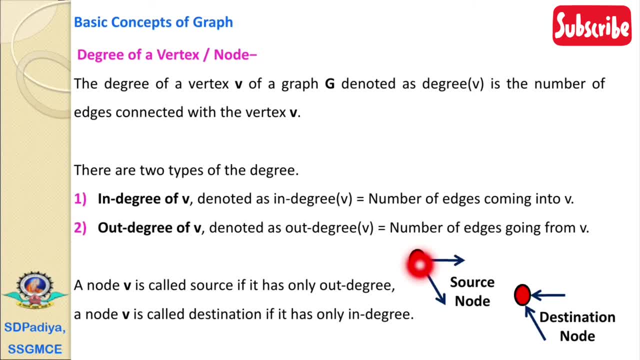 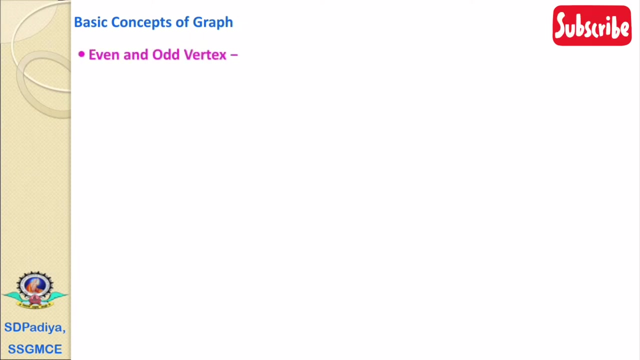 it has only out degree and zero in degree. therefore it is called as source. and for the second node there are only two incoming edges, means it has only in degree but zero out degree. therefore it is considered as the destination node. Now we will discuss about the type of vertex. there are the two types, called as even vertex. 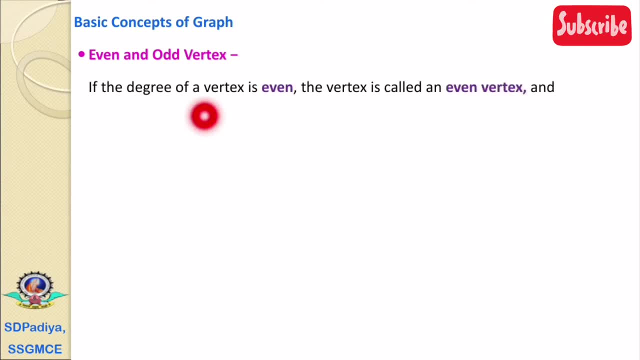 or odd vertex. If the degree of vertex is even, then the vertex is called an even vertex and the degree of vertex is odd, Then the vertex is called an odd vertex. The next is a degree of a graph. The degree of a graph is the largest vertex degree of that graph. 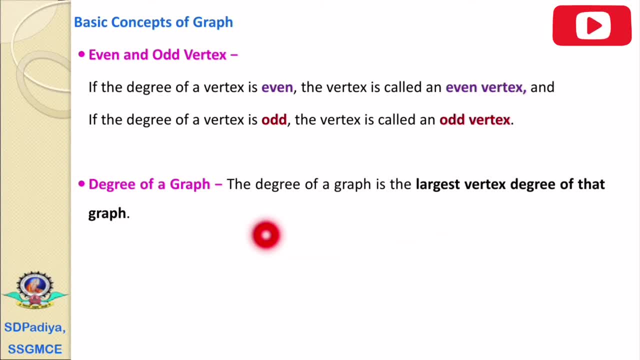 For example, if we have the three vertices in a graph ABC, the degree of A is 3,, degree of B is 4 and degree of C is 5, then degree of a graph is a 5.. Suppose a largest vertex degree of that graph that is 5.. 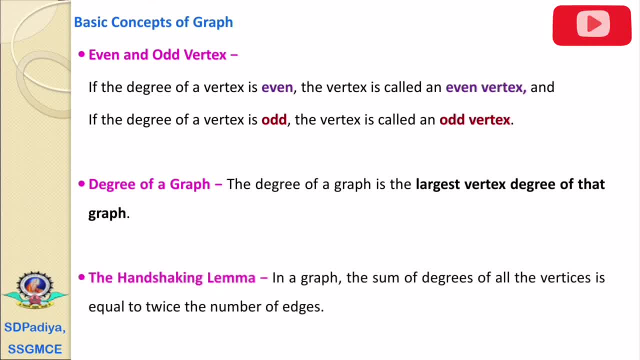 The next is the handshaking lemma. In a graph the sum of degrees of all the vertices is equal to twice the number of edges. If suppose in any graph we have the 10 edges, then the sum of degree of all the vertices is equal to twice. 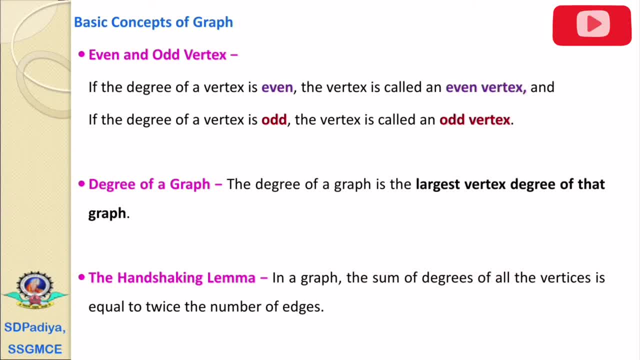 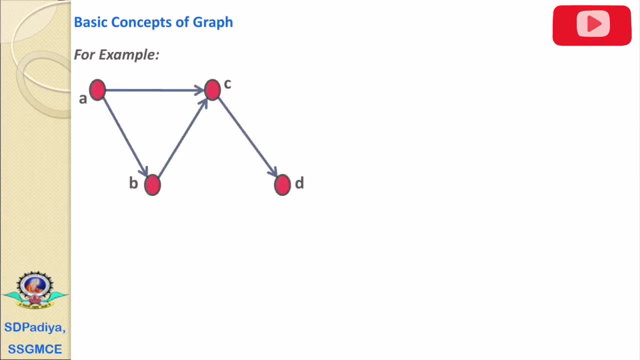 That is, the sum of the degree of all the vertices is equal to 20.. If in a graph we have 15 number of edges, then the sum of the degree of all the vertices is equal to 30.. We will take one example now. in this example we have 4 vertices ABCD which are connected. 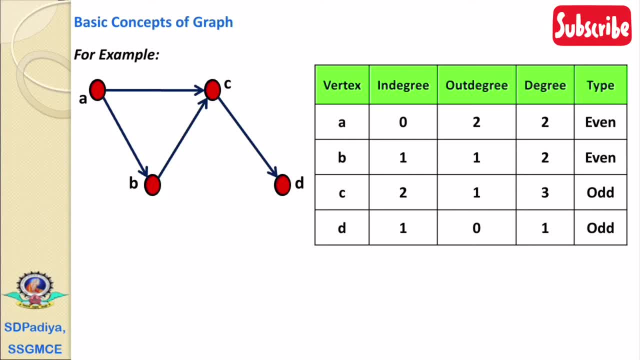 with the 4 edges And these edges are directed edges, That is, edge from A to B, edge from A to C, edge from B to C and edge from C to D. Now to find out the in-degree, out-degree, the total degree and type of a vertex, we 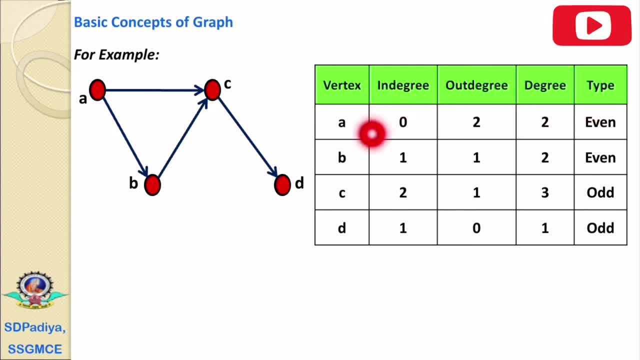 have designed one table here for the vertex A, vertex B, vertex C and vertex D. Now we will start from the first vertex A. At a vertex A, there is no any incoming edge, therefore in-degree 0. And there are 2 outgoing edges, A to C and A to B. Therefore out-degree is 2.. 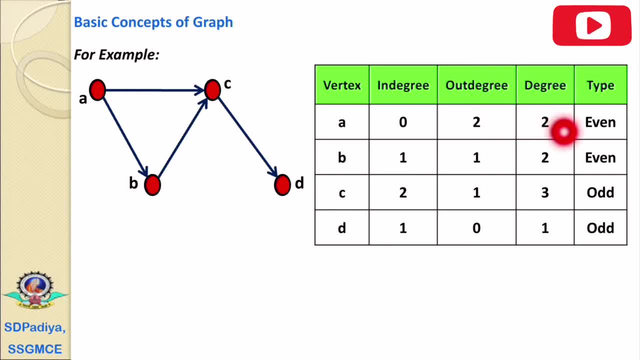 In-degree 0 and out-degree 2. therefore total degree it is 0 plus 2, that is equal to 2.. 2 is even. Therefore, type of a vertex is even. So we have 2 out-degrees. So we have 2 out-degrees. 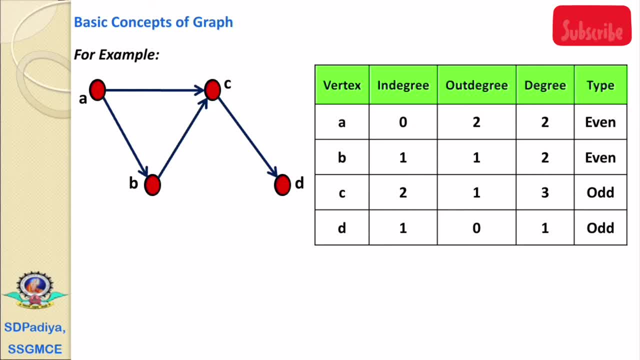 So we have 2 out-degrees, even vertex same for the second vertex, b b. it has one incoming h that is a to b, and one outgoing h that is b to c. therefore in degree is 1 and out degree is 1, 1 plus 1. therefore total degree is 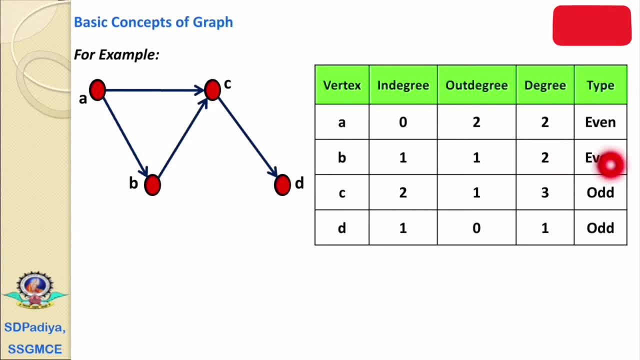 equals to 2. 2 is even. therefore its type is even vertex. next for a vertex: c, c. it have two incoming edges, a to c and b to c. therefore, in degree for c is 2 and it has one outgoing h, that is, c to d. 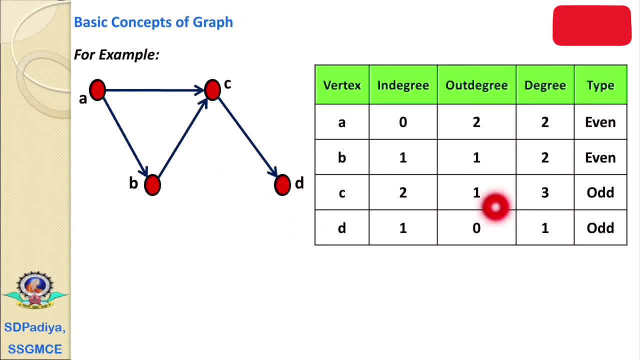 therefore, out degree is 1, 2 plus 1, total degree is 2 and it has one outgoing h. that is c to d. therefore out degree is 1, 2 plus 1. total degree is 3. 3 is an odd number, therefore c, it is a odd vertex. for the last vertex, d. 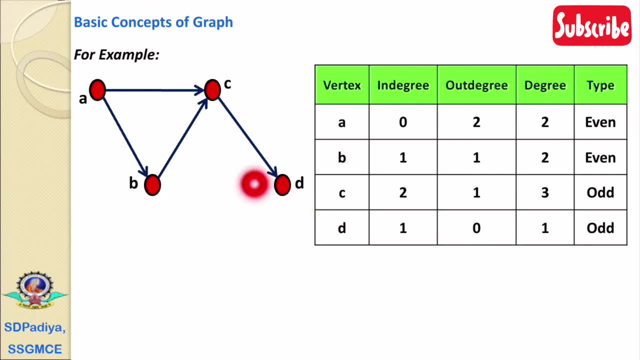 it has only one incoming h, that is c to d, and there is no any outgoing h. therefore, for the vertex d, in degree is 1, out degree 0 and total degree 1 plus 0 is 1. therefore d is a odd number, therefore c, it is a odd vertex. for the last vertex, d, it has only one incoming. 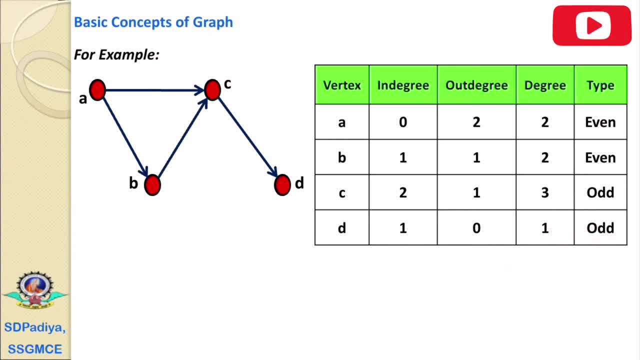 h, that is c to d. therefore it is odd vertex. now, if in a graph there is a, any node which has only the out degree, that's we called a source and which has only the in degree, that's we called destination. now, in this graph, if we observe a vertex a, it has only the out degree. therefore, 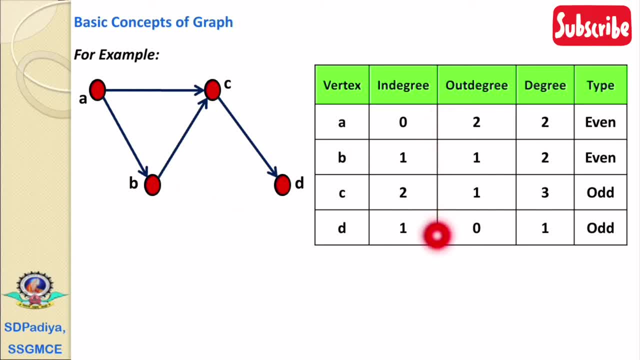 it is called a source node, and there is a vertex d and there is a out degree. therefore it is called a destination node. if we observe a vertex d which has only in degree, out degree is 0. therefore vertex d is called destination node. now here vertex a, its 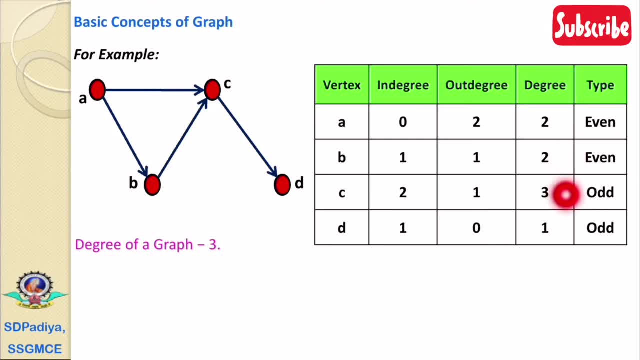 degree is 2. vertex b degree is 2. vertex c- it's a degree is 3 and for the vertex d the degree is 1. the highest degree of a vertex is 3. therefore 3 it will end up as a points here in the MyR. 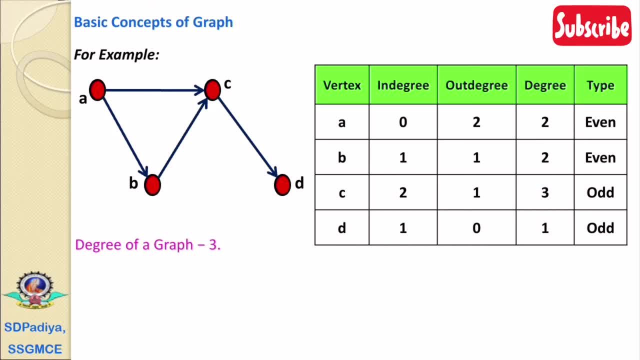 made of z symbols and this is a node which coordinates between theotecs d AND theodecs iniendo laughing, a degree of a graph, The sum of degree of all the vertices, that is 2 plus 2 plus 3 plus 1, it is equals to 8.. We have already discussed that node A. it has only outgoing edges. it. 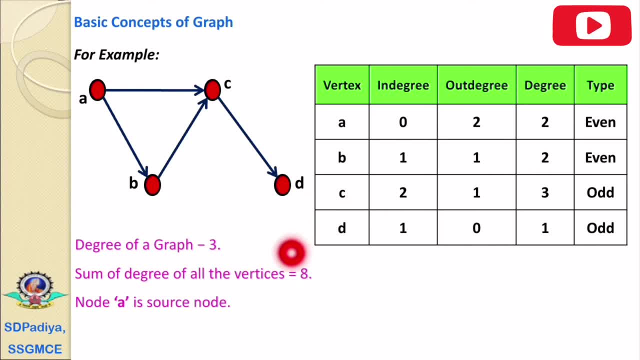 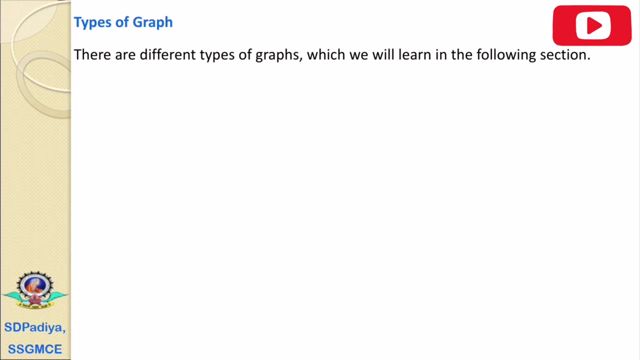 has only out degree, 0 in degree. therefore, node A is considered as a source node and the node D. it has only incoming edges, that is, in degree but 0 out degree. therefore, node D is considered as a destination node. Now the next topic is types of graph. There are 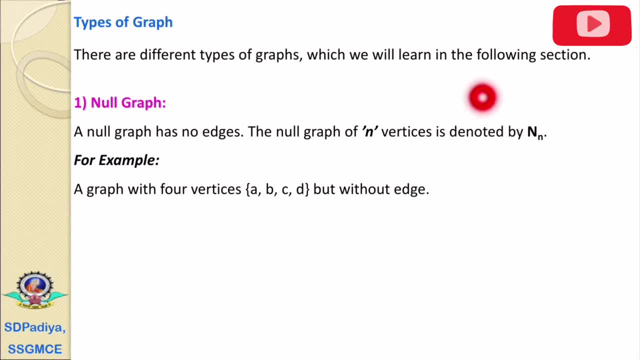 different types of the graphs, which we will learn in the following section. The first type is a null graph. A null graph has no edges. The null graph of the n vertices is denoted by the capital N, suffix the small m, that is. 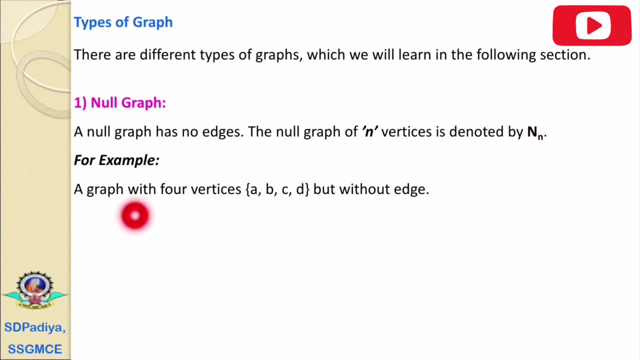 number of vertices in a graph. A graph with 4 vertices- A, B, C, D, but without edge. that's we called a null graph. The null graph may have a single vertex, 2 vertices, 3 vertices, up to n number of vertices, but without edge, that's we called a null graph. 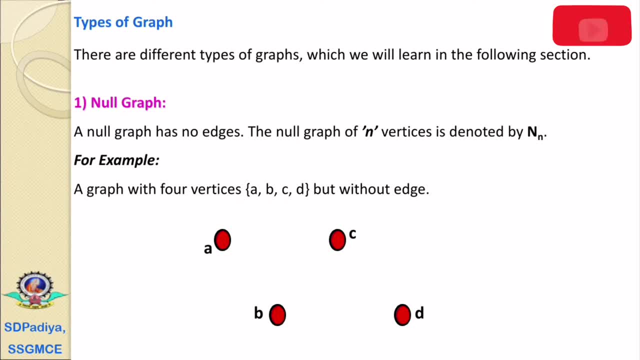 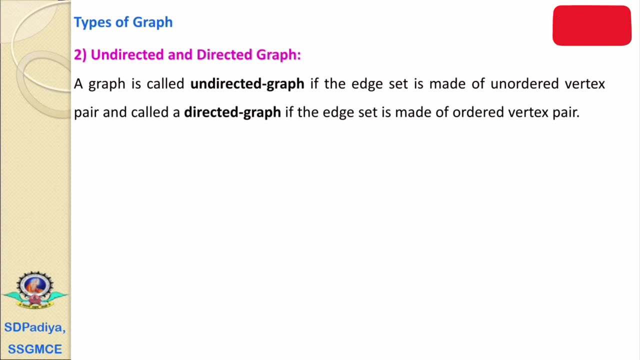 Now in this example we can clear there are 4 vertices, A, B, C, D, but there is no any single edge. Therefore it is called a null graph. The second type is based on the availability of the direction. This type is undirected and the directed graph If in a graph to the 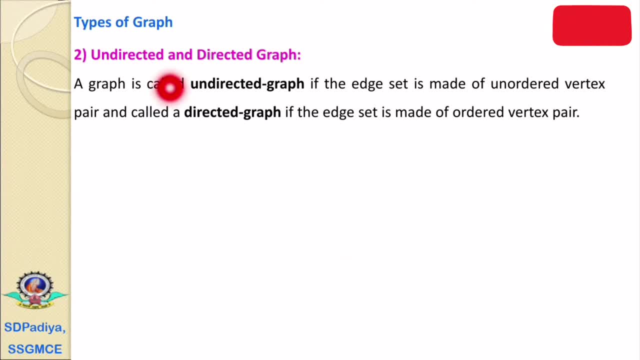 average edge there is no direction, then it is called a null graph. The second type is based on the availability of the direction. Therefore it is called undirected graph. And if in a graph to the all edges the direction is defined, then it is called directed graph. 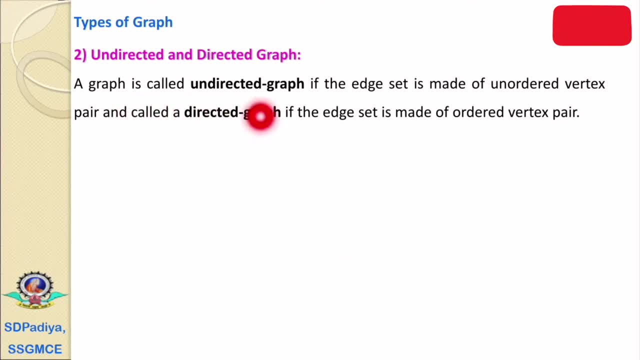 We'll see. theoretically, a graph is called undirected graph if the edge set is made up of unordered vertex pair And called a directed graph if the edge set is made up of the ordered vertex pair. If a graph is undirected, then it will be an unordered vertex And if it is a directed. 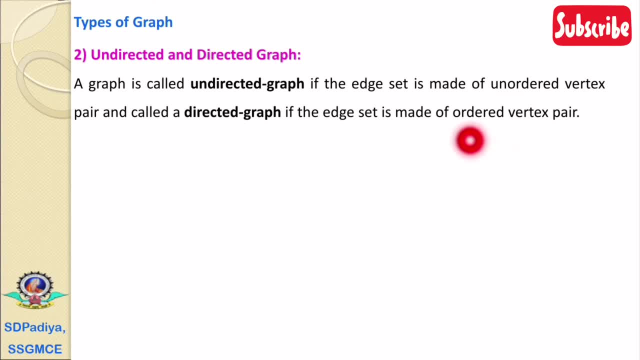 graph. there is an importance to the order. Therefore it will be the ordered vertex pair. In undirected graph we can consider any edge from A to B, then B to A also, But in ordered pair, if there is a pair A to B, Then we can also consider any edge from A to B. But in 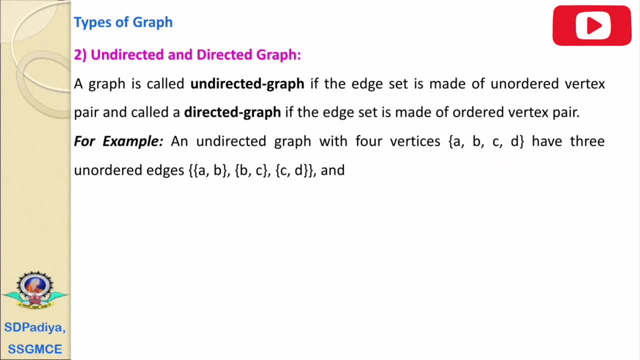 undirected graph, we cannot consider it as a, B to A. Let's have the example that an undirected graph with the four vertices ABCD have three unordered edges: the A, B. Then we can consider it also the B A. The second is B C Also. 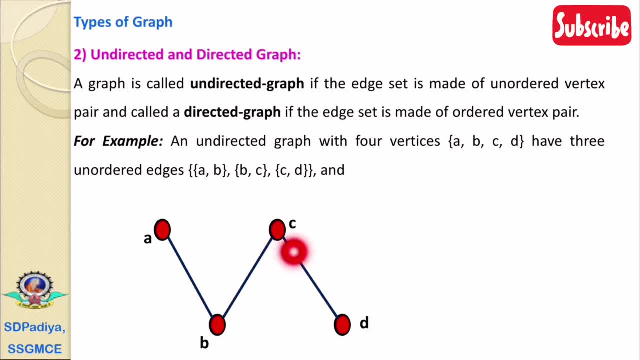 consider as a C, B. Third is C D, That's we can also consider as a D, C. Therefore, all three pairs are defined as a set. in the curly braces That means it is unordered, And unordered means it is undirected graph. 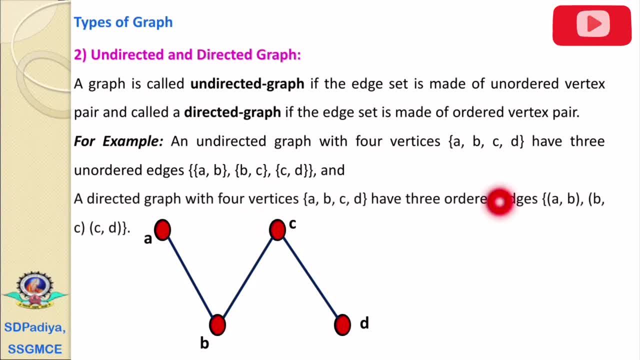 We have again one example here for the directed graph. A directed graph with the four vertices ABCD have three ordered edges. the first is A B. Now we cannot consider it as a B A. Second is B C. third is the C D. For the directed graph there are the ordered pairs, Therefore these: 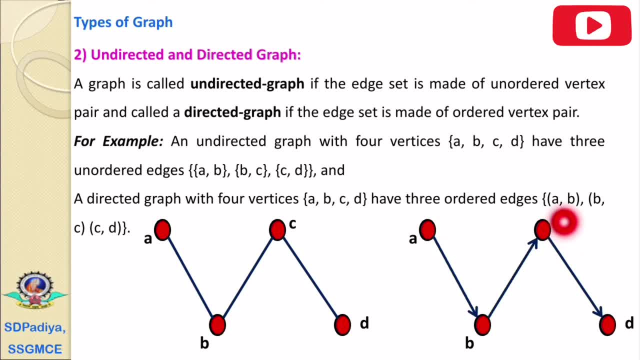 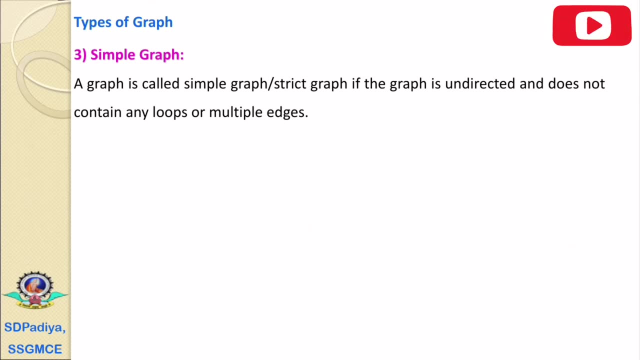 three edges are defined in the parenthesis: for the ordered pairs And for unordered pairs. these edges are defined as a set in the curly braces. Third type is a simple graph. A graph is called a simple or the strict graph if the graph is undirected and does not contain any. 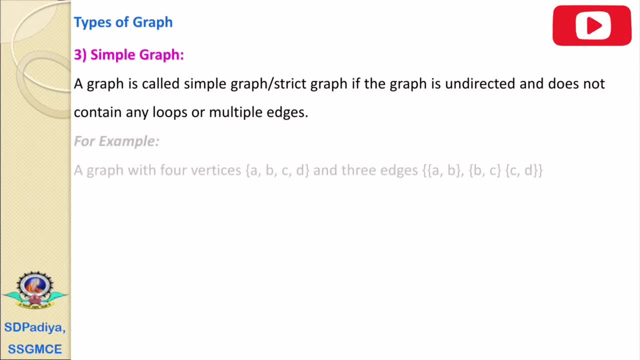 loop or the multiple edges Means if in a graph there is no loop or the multiple edges, then it is called as a simple graph. Let's have the again example that a graph with the four vertices A, B, C, D and the three edges A, B, B, C. 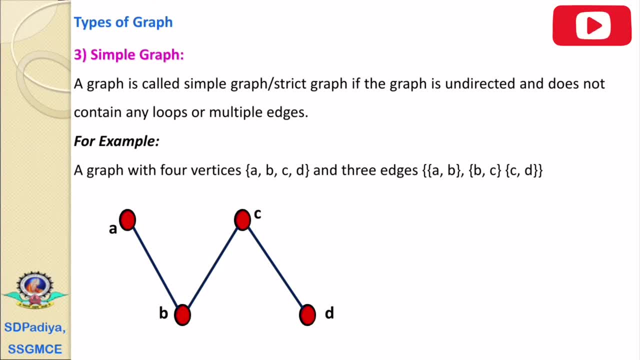 C, D. Now in this graph there is no any loop between the any two nodes or there is no any multi lines, multiple edges between any two nodes. Therefore we can say this given example is a simple graph. Let's have the second example again Now in this example, also between the any two. 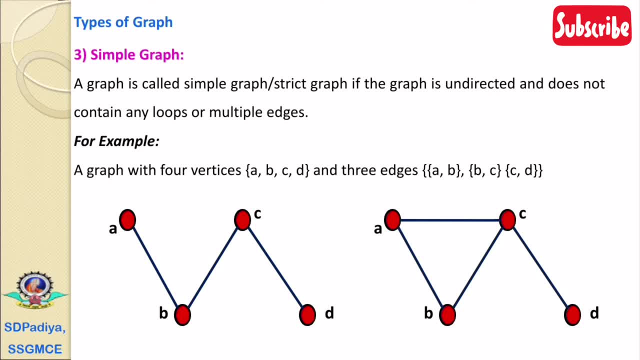 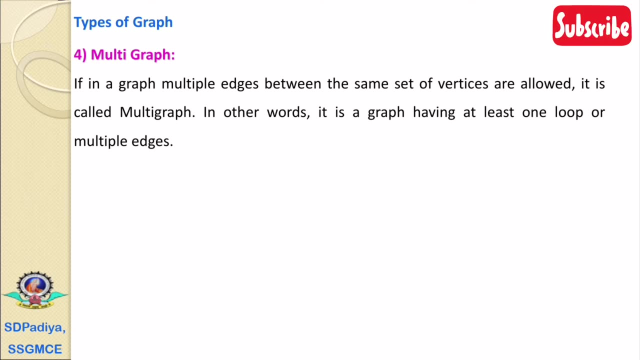 nodes. there is no any loop or The multiple edges and it is undirected also. Therefore it is also an example for simple graph. The fourth type of a graph is multigraph. If in a graph multiple edges between the same set of 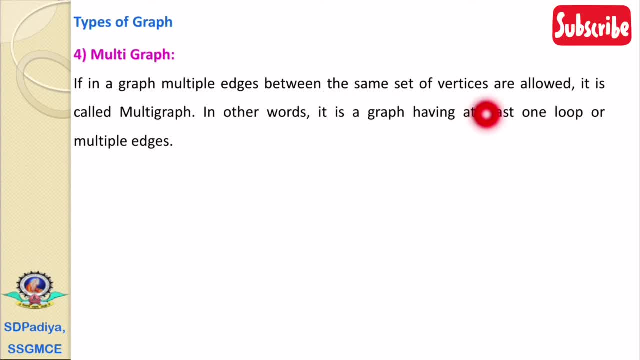 vertices are allowed or are available, then it is called multigraph. In other words, it is a graph which contains at least one loop or multiple edges. Means if in a graph between any two nodes there is a loop or multi edges are available, then it is called as a multigraph. Let's have an example. 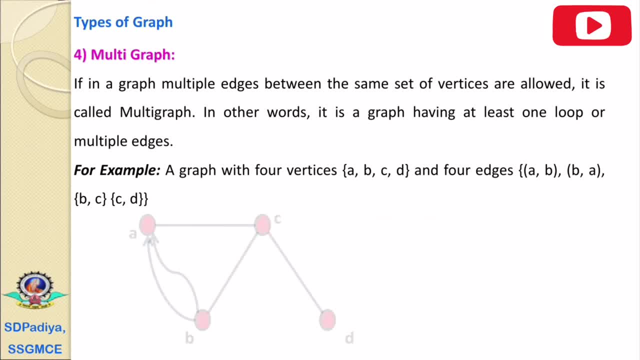 a graph with the four vertices A, B, C, D and the four edges: the A, B, B A, B, C and C D. First we will have the example where there are the two edges from B A. 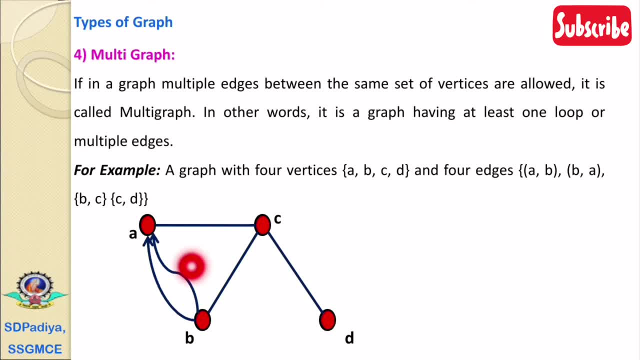 Now you can observe in the graph, two lines, two edges are available with the same characteristics, with the same meaning, That is B, A. Then this graph is called a multi-graph. In the second example now we can observe there are the two edges with the same characteristics, that is A to B. 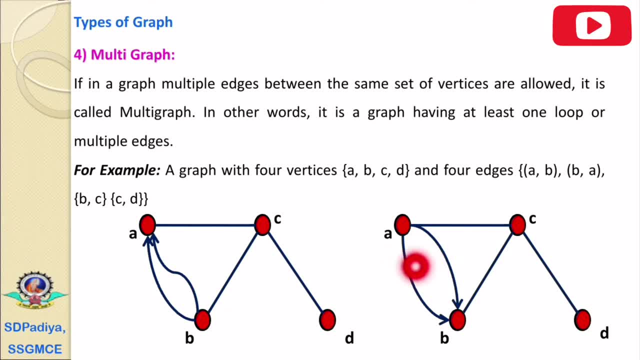 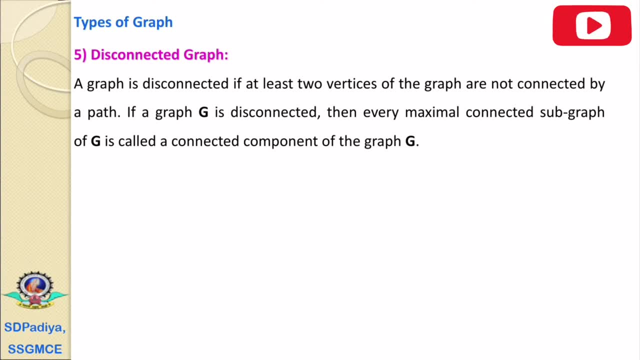 Now the meaning of both edges is same. Therefore it is called a multi-graph. The next fifth type of the graph is disconnected graph. If we can divide the any graph into the two sub-graphs, then we called it a multi-graph. 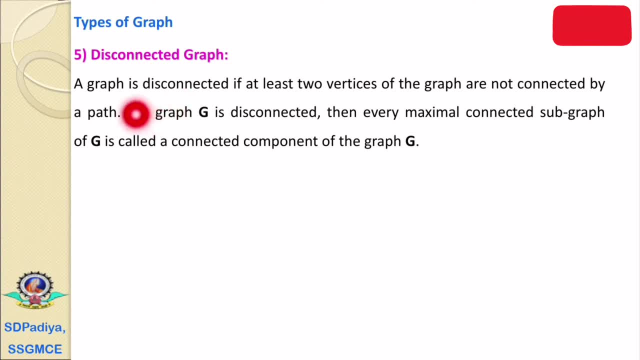 Then it is a disconnected graph. Let's have: a graph is disconnected if at least two vertices of the graph are not connected by a path. If a graph which is denoted as a capital G is disconnected, then the every maximal connected sub-graph of the G is called a connected component of the graph G. 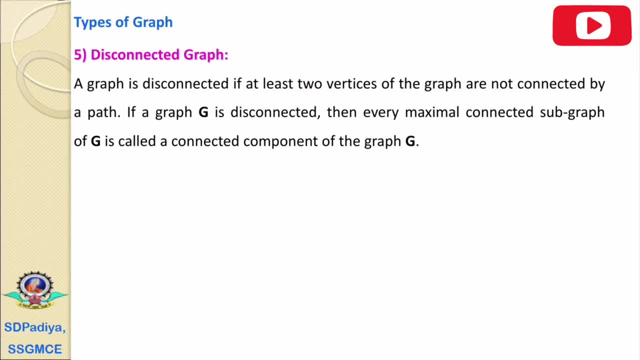 Means if the any graph can be divided into the two sub-graphs, then it is called a disconnected graph. If we have the example, a graph with the four vertices- A, B, C, D and only the two edges, that is, A to B and the C to D. 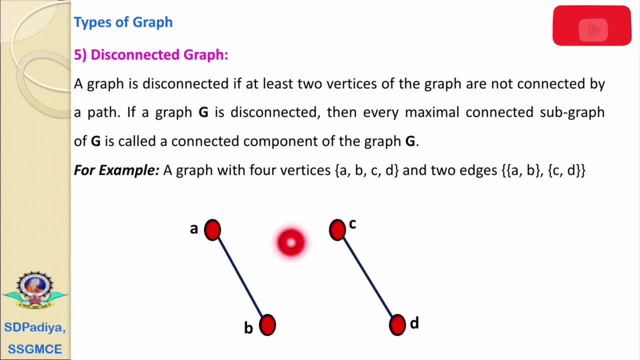 Now it is a single one graph with the four vertices, But now we can divide this graph into the two sub-graphs, One as a A, B and second as a C, D. Therefore it is considered as a disconnected graph. Next is connected graph. 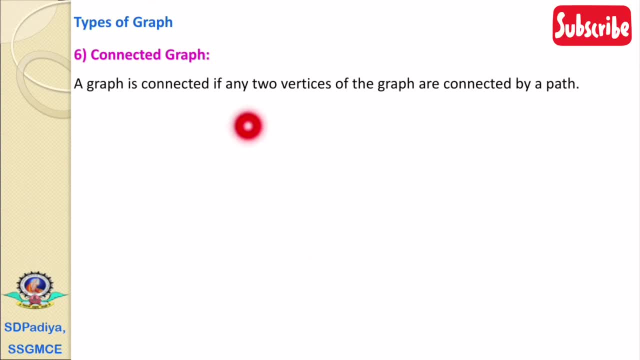 A graph is connected if any two vertices of the graph are connected by a path. Now there are two types of connected graph. First is called strongly connected And second is called weakly connected graph. A graph is said to be strongly connected if for any pair of nodes of the graph, 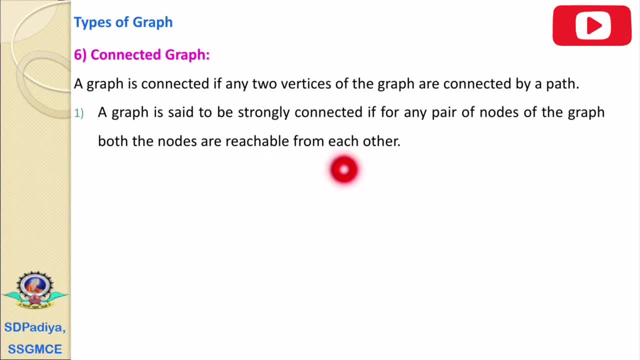 both the nodes are reachable from each other. Let's have the example: If we have the graph like that with the two vertices A- B, the first is for the undirected and second is an example for directed. Now if we observe in the first, A is reachable from the B and B is also reachable from the A, 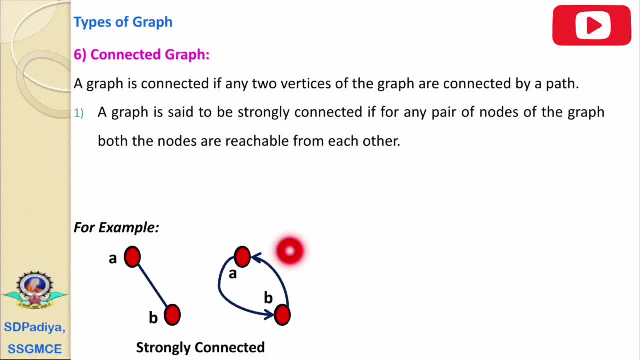 because it is undirected. And in the second directed graph, again, node A is reachable from the B and B is reachable from the A. That is, if in a graph for any two pairs of the nodes, both the nodes are reachable from each other. 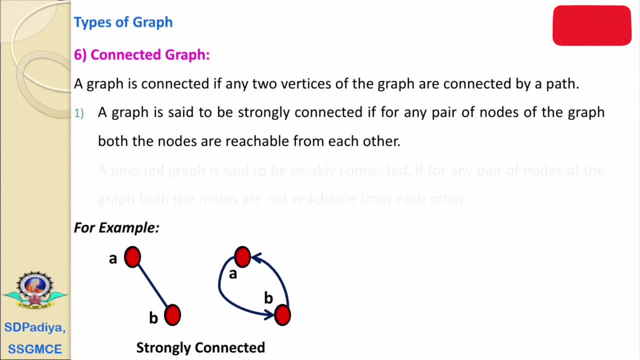 then it is called strongly connected graph. The second is a weakly connected. A directed graph is said to be weakly connected if, for any pair of nodes of the graph, both the nodes are not reachable from each other. Let's have the example. 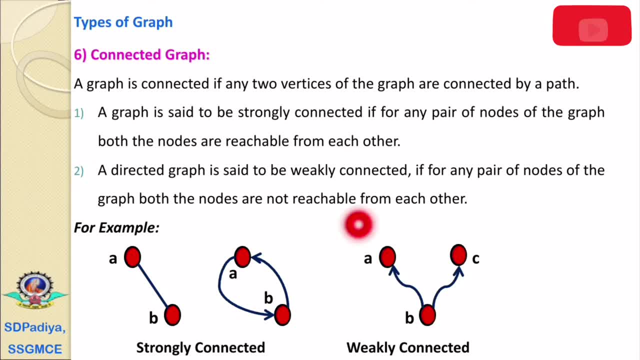 Now in this graph, A is reachable from B, C is reachable from B. Yes, But for a pair of A and C. if we consider a pair of A and C, then A is not reachable from C and C is also not reachable from A. 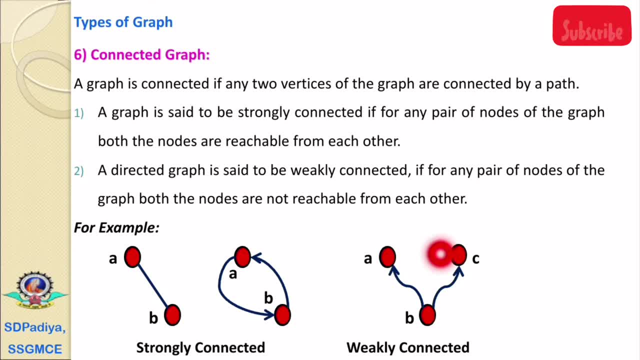 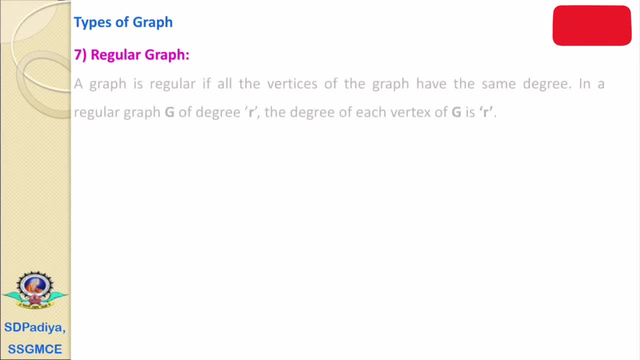 Therefore we call it is weakly connected. graph Seventh is regular graph. A graph is regular if all the vertices of the graph have the same degree. In a regular graph G of degree R, the degree of each vertex of G is R. 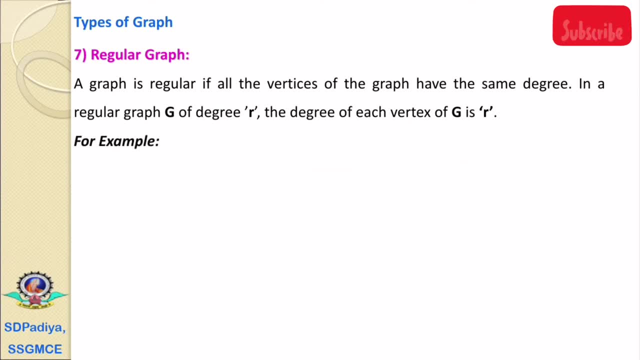 Means. in short, if in a graph the degree of all the vertices is equal, it is the same, then it is called as a regular graph. Now again we have the example A graph with the four vertices A, B, C, D and the four edges, like the A to B, A to D, B to C and C to D. 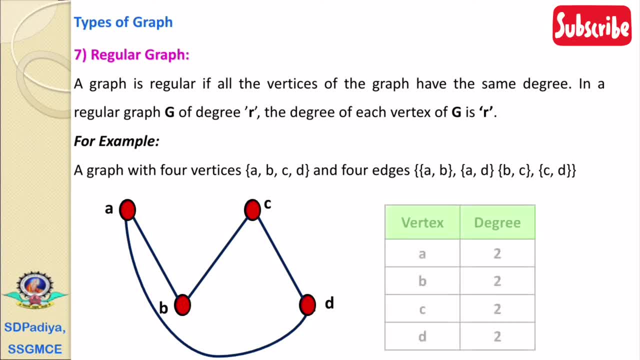 Now, if we check the degree of the vertex A is 2,, the degree of a vertex is 2, degree of a vertex is 2, and degree of vertex D: it is also 2.. The number of edges connected to the vertex. 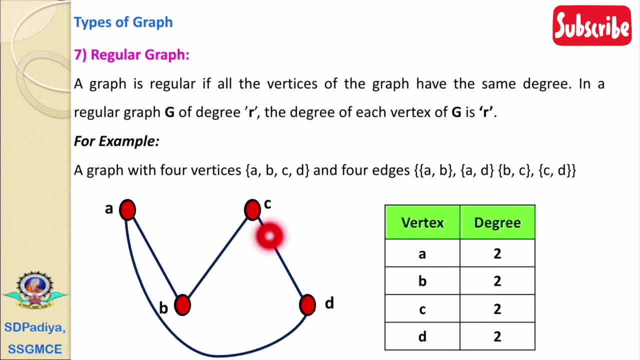 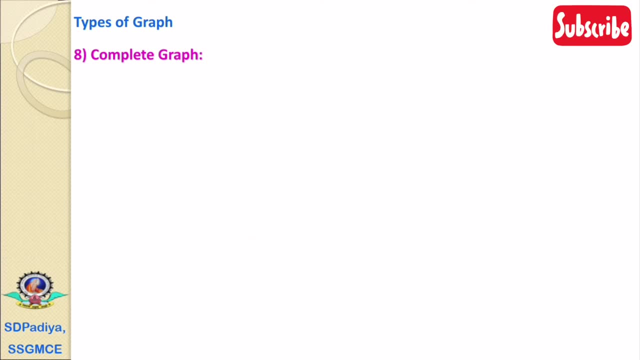 that's we call a degree of a vertex. Now in this graph all the vertices A, B, C, D have the same degree, that is, 2.. Therefore this graph is called as regular graph. Next is a complete graph. 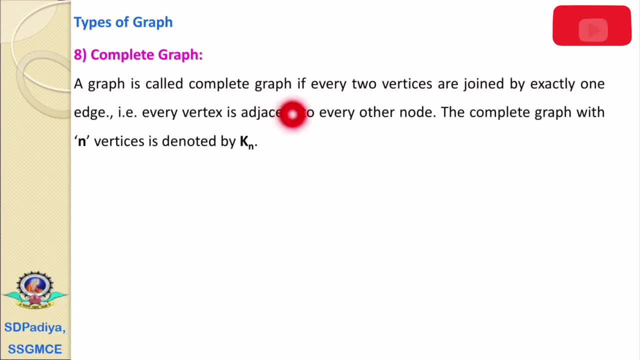 A graph is called complete graph if every two vertices are joined by X. exactly one edge, that is, every vertex, is adjacent to every other node. The complete graph with N vertices is denoted by the K suffix N If in a graph, for any pair of any two nodes there is a direct edge. 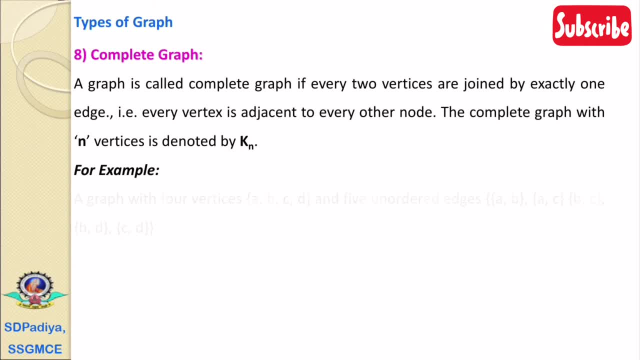 then it is called a complete graph, For example, a graph with the four vertices A, B, C, D and the five unordered edges, that is, A, B, A, C, B C, B, D, C, D. 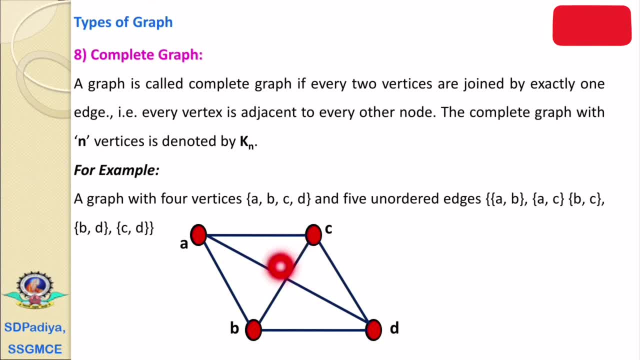 then it is called a complete graph. There must be a sixth edge, that is the A D. Now if we check for this graph, between any two nodes there is a direct edge. Therefore it is considered as a complete graph. 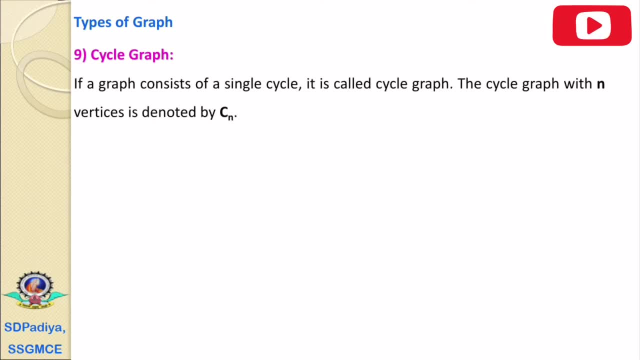 Next is a cycle graph. We know the meaning of cyclic. If a graph consists of any single cycle, then it is called a cycle graph. The cycle graph with N vertices is denoted by the capital C for the cycle. capital C suffix small n. 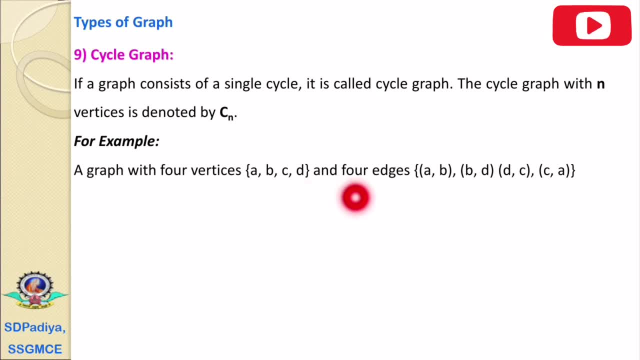 A graph with four vertices: A, B, C, D and the four edges, the A, B, the B to D, D to C and C to A. Then now in this graph, if we start from any node, then we can reach to this node. 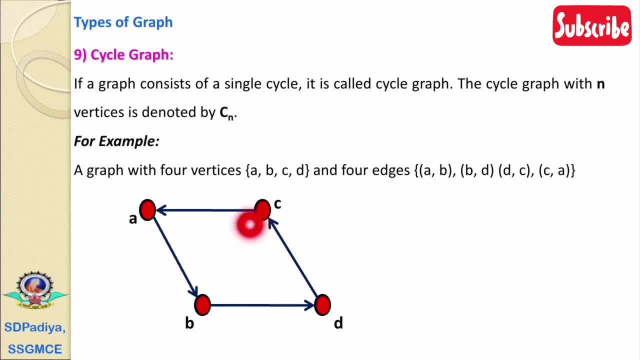 If we start from the node C, then we have a path from C to A, A to B, B to D and again. D to C Means any node is reachable from itself. Therefore we call it is a cycle graph. Next is weighted graph. 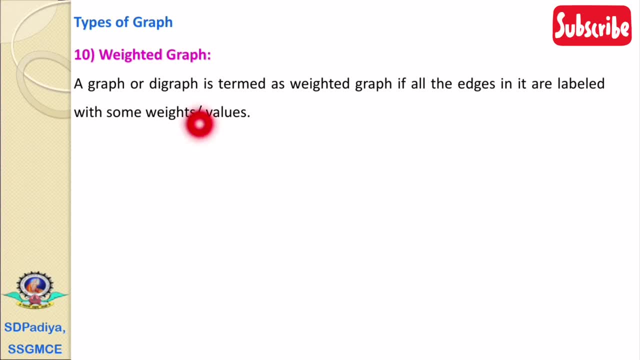 The weight means a value. A graph or digraph that is, a directed graph is a term as a weighted graph if all the edges in it are labeled with the sum weights or the values. Generally, these weights or values are used for the distance between the any two points. 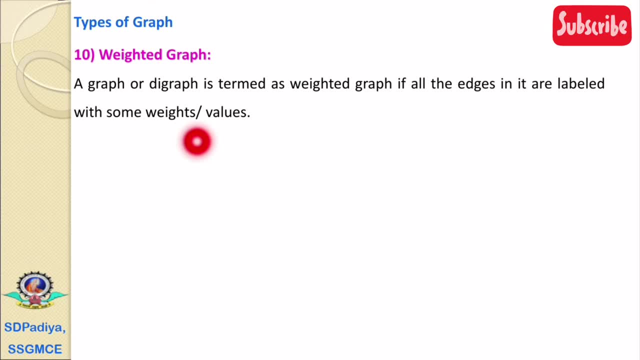 the distance between the any two nodes, or we can use the any different values. Let's have the example A graph with the four vertices. Suppose for the four places A, B, C, D and the four edges as the four roads connecting roads. 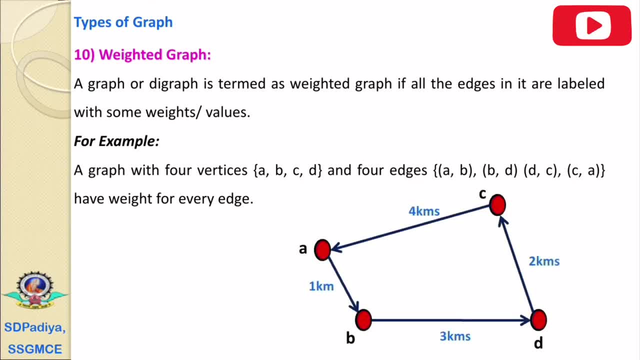 that is, A to B, B to D, D to C and C to A have a weight for every edge. that is a distance. The C to A: it has a four kilometer distance. The A to B: one kilometer distance. 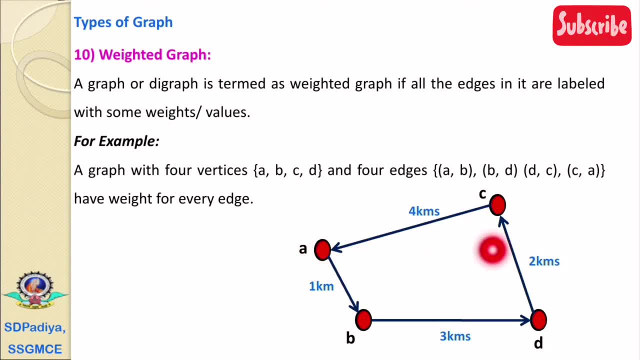 B to D it has a three kilometer distance and D to C it has a two kilometer distance. A graph in which to the every edge there a value is defined. then it is called a weighted graph. Next, here the distances between the four places are shown in the kilometers. 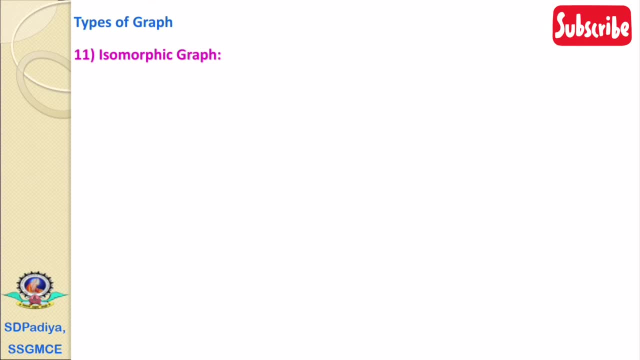 The eleventh type of the graph is the isomorphic. Before that we have seen, the morphic means a mapping, That is we call the morphism. The two graphs are the isomorphic if there exists a one-to-one correspondence between the nodes of the two graphs. 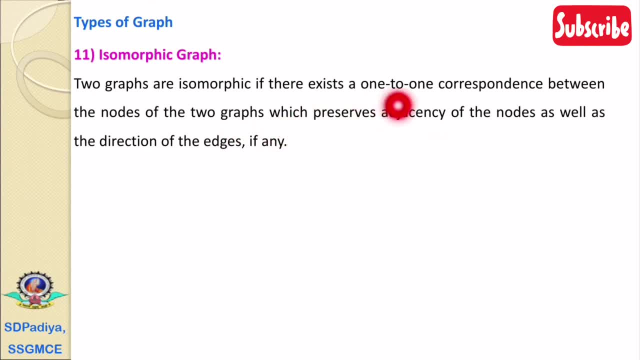 To understand about the isomorphic, or what do you mean by the one-to-one correspondence? you can refer a video on the functions in the discrete mathematics. We have already prepared a separate video on the discussion of one-to-one correspondence and the morphism. 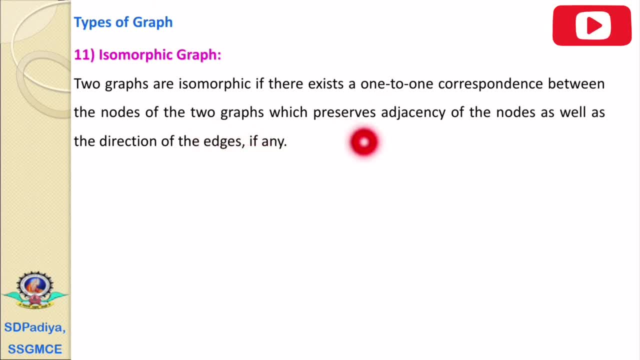 Now here the two graphs, which preserves the agency of the nodes as well as direction of the edges, that's we call the isomorphic graph. According to the definition of isomorphic, we note that any two nodes in a one graph which joined by an edge, 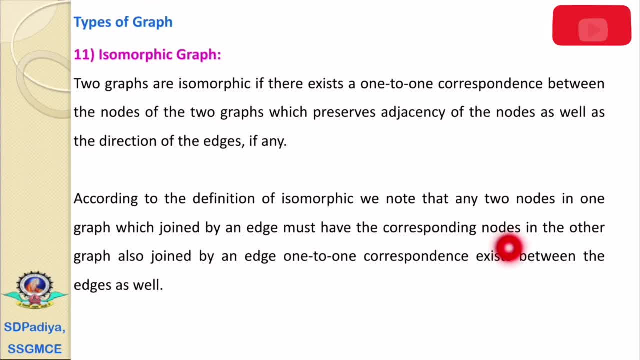 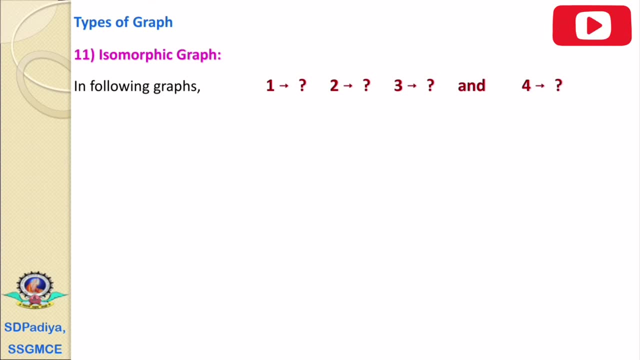 must have corresponding nodes in the other graph also Joined by an edge. one-to-one correspondence exists between the edges as well, Means if we have two graphs and in between this two graphs the every vertex has it's same vertex in the other graph. 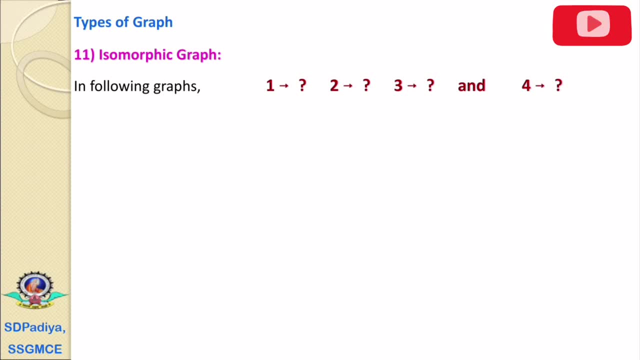 or vertex with the same characteristics in the other graph, or vertex with same characteristics in the other graph, or vertex with the same characteristics in the other graph, in the other graph, then we call: these two graphs are isomorphic. Now we have an example. 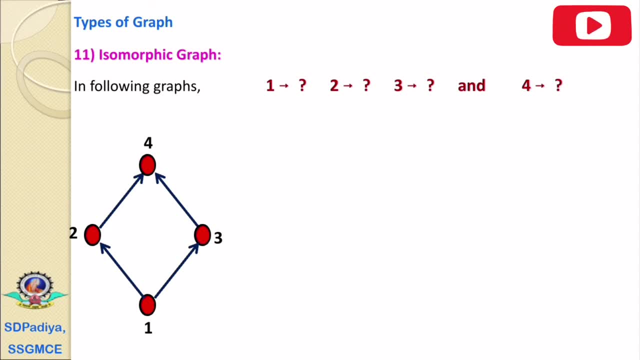 Suppose, in a first graph there are four vertices: 1,, 2,, 3, 4.. Now if we have a second graph with the four vertices A, B, C, D, then how we can define: these two graphs are isomorphic graphs. 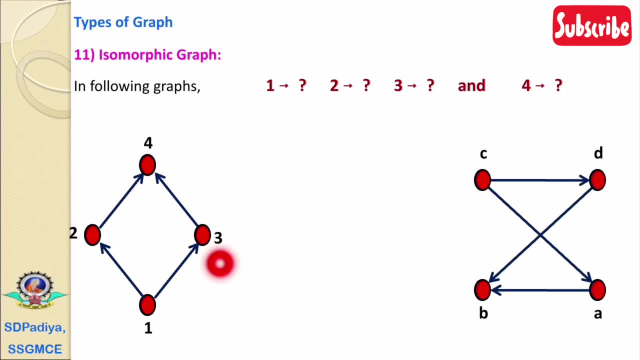 In this first four vertices, 1,, 2,, 3, 4, how the characteristics? the characteristics based on the incoming degree and outgoing degree, that is, in degree and out degree. Now we will check one by one. The vertex 1, it has the two out degrees: 0 in degree. Vertex 2, it has 1 in degree, 1 out degree. 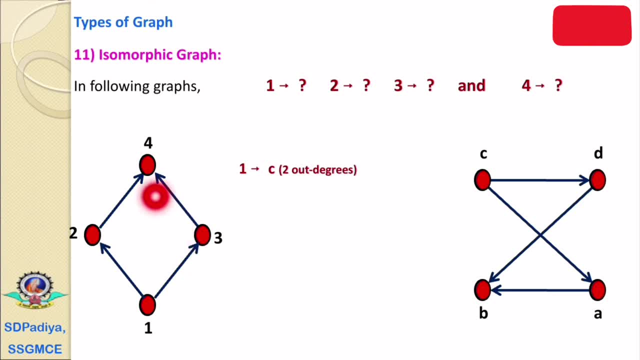 Vertex 3, it has 1 in degree, 1 out degree, and vertex 4, it has 4 in degree, 0 out degree. Similarly, in a second graph, the vertex A, it has 1 in degree, 1 out degree. 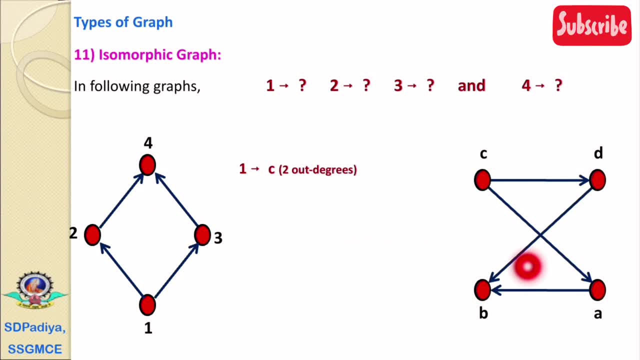 Vertex B, it has 2 in degree, 0 out degree degree. vertex C: two out degrees, zero in degree. and vertex D, one in degree, one out degree. Therefore, by mapping the vertex with the same characteristics, we have defined that A1 have a same characteristics as a vertex C in a second. 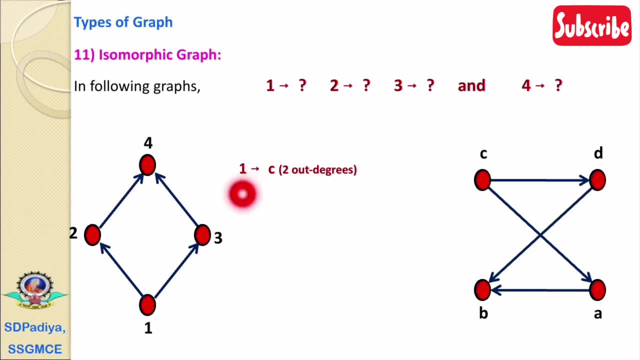 graph. that is, in a first, vertex 1 and in a second, vertex C. both have the zero in degree and two out degree. therefore these two are with the same characteristics. Second is a vertex 4 in first and vertex B in second. both has the zero- zero in degree- and. zero in one degree. So by mapping A3 out degrees, Jesus can see how these dá starring, an indication that those two acontecendo. Gut fingers to this Tang Ge하시는 line. in case of the VISont to orient in it is a. 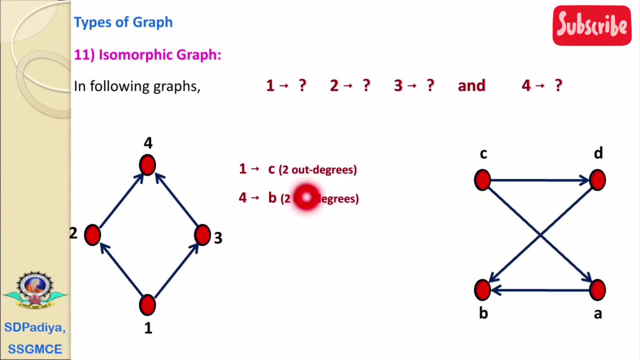 out degree and 2 in degree. Therefore the B is considered as a 4.. The next is an example: the vertex 2 and the vertex A both has a 1 in degree and 1 out degree. and the next is the vertex 3 and the vertex D: both has again the 1 in degree and 1 out degree. Therefore, 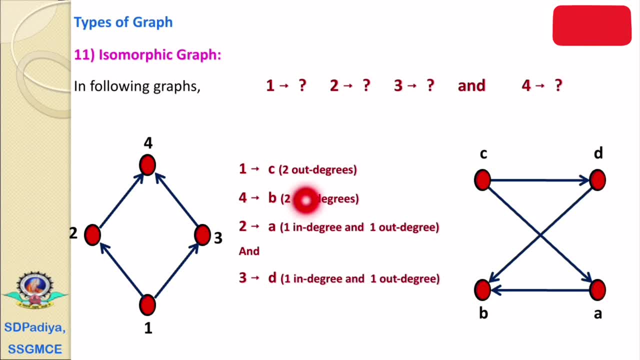 we can define that these two graphs are isomorphic graphs. There is an equivalent vertex in a second graph for the vertex in a first graph, The 1. it has an equivalency with the C. 2. it is equivalent to the B vertex 4. it is equivalent to the B vertex 2. it is equivalent. 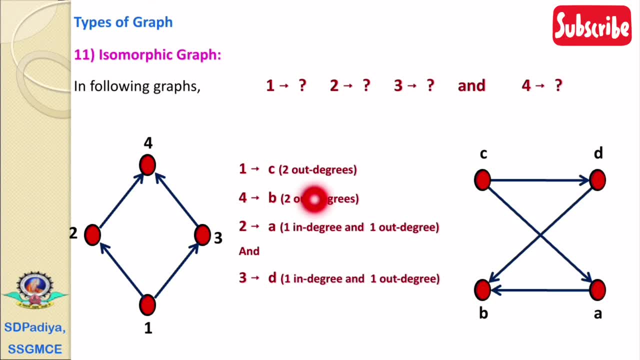 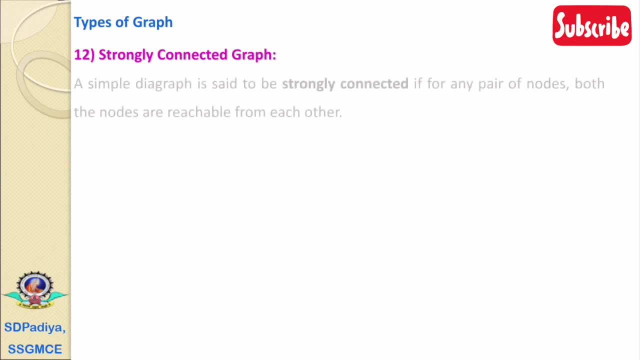 to the node A and vertex 3 it is equivalent to the node D. Next twelfth type is a strongly connected graph. We have already covered before that a simple diagraph is said to be strongly connected if, for any pair of nodes, both the nodes are. 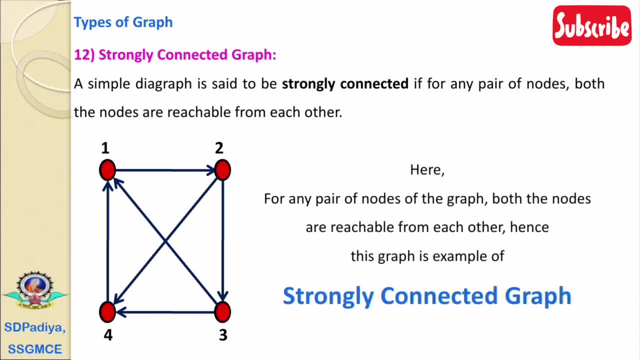 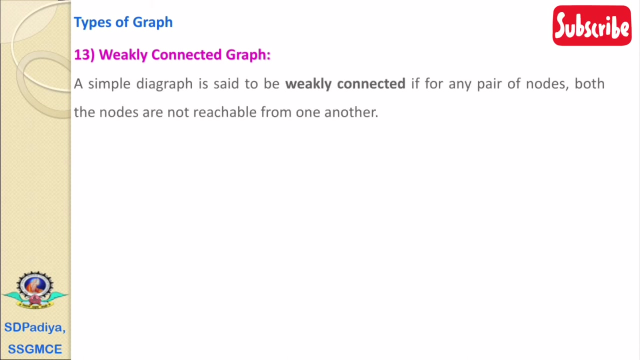 reachable from each other. Now here we can check for any pair of any two nodes. both the nodes are reachable from each other. Therefore this graph is called as a strongly connected graph. Next type is weakly connected graph. A simple diagraph is said to be weakly connected if 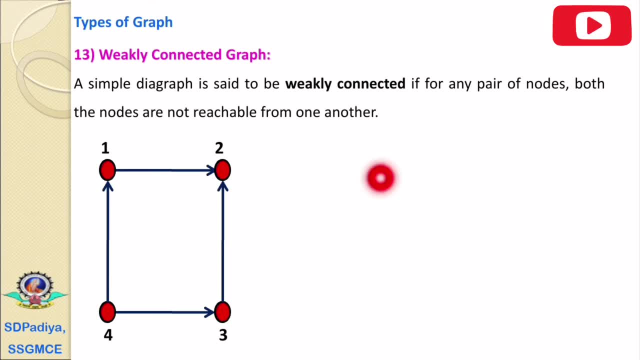 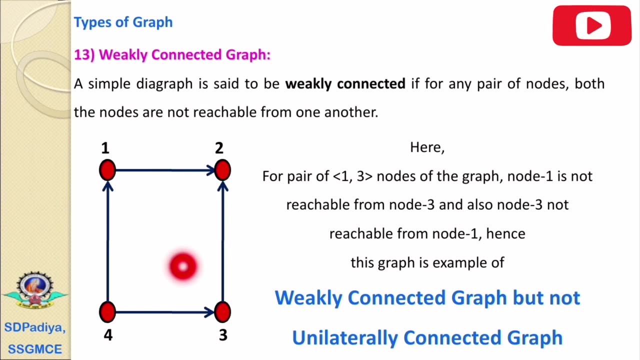 for any pair of nodes in the graph. both the nodes are not reachable from each other. Now here, if we check for a pair of nodes 1 and 3. Then we cannot reach at the 1 from the 3 and we cannot reach at the 3 from the 1. That 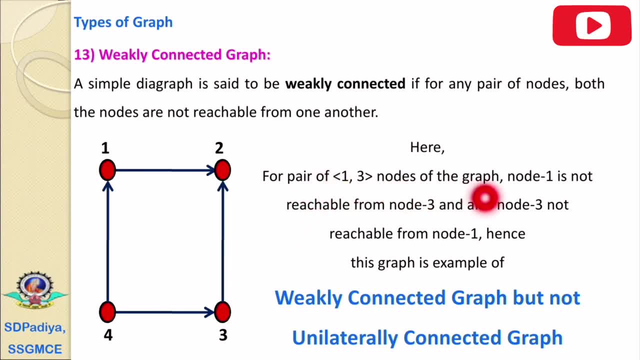 is for a pair of 1,3 nodes of the graph. node 1 is not reachable from node 3, and also node 3 is not reachable from node 1.. Hence this graph is called the weakly connected graph, But not a unilaterally connected graph. 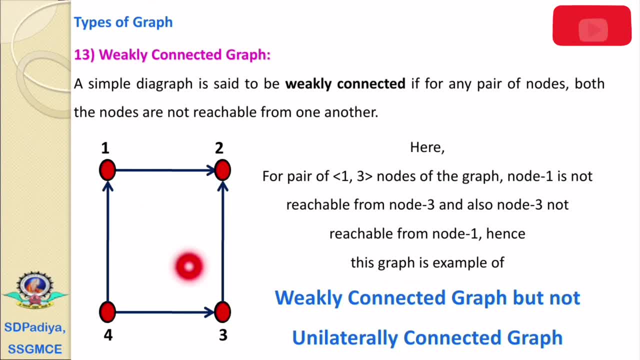 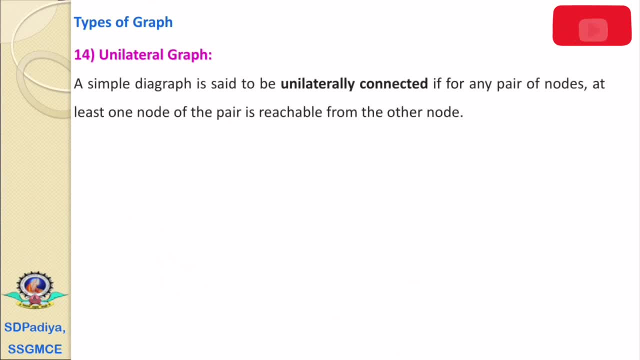 Next is a unilateral graph. Here is the unilateral graph. The uni means one, A simple diagraph is said to be unilaterally connected if, for any pair of nodes, the atleast one node of the pair is reachable from the other node. Let's have the example. 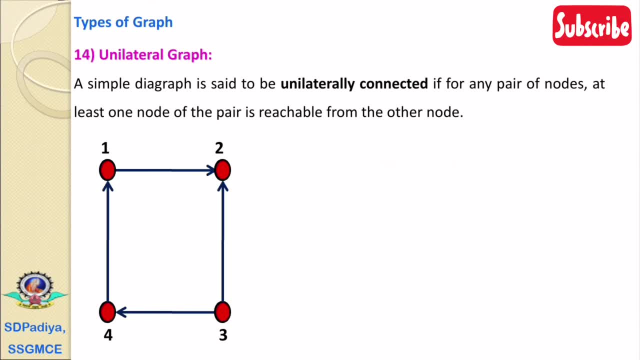 Now in this graph, If we observe, for every pair will start from the pair of 1 to 2, then there is a relation from 1 to 2, but not 2 to 1. We cannot reach at the 1 from the 2 because 2 it does not has outgoing age. 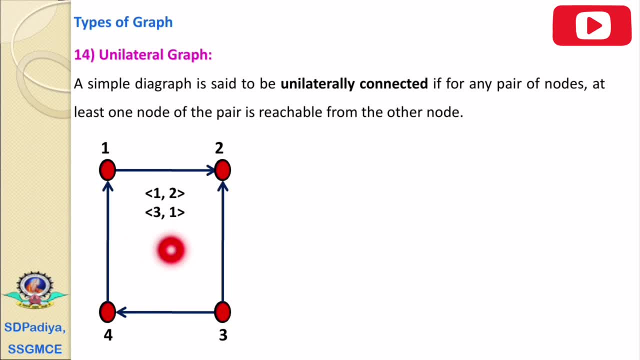 The second is a pair of 1 to 3.. Now here we can reach from the 3 to 1, that is, 3 to 4 and 4 to 1.. Through this path we can reach at the 1, that is, there is a path from 3 to 1, but there is. 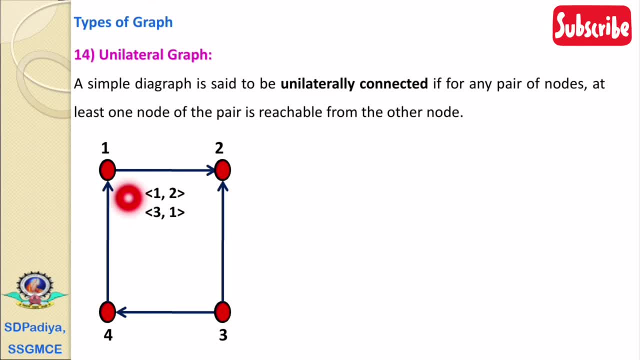 no path from 1 to 3.. There is no any path from 1 to 3.. The next is for a pair of 4 comma 1.. The 4 comma 1: there is an direct age, But there is no direct age. 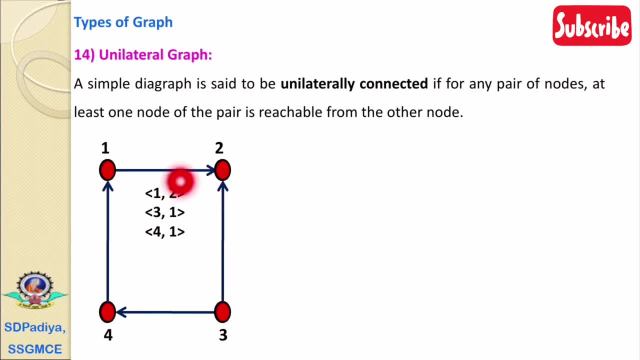 There is no any path from 1 to 4.. There is no any path from 1 to 4.. Next is for a pair of 3 and 2. The 3 to 2: there is an direct age, but there is no any path from 2 to 3 because 2 does. 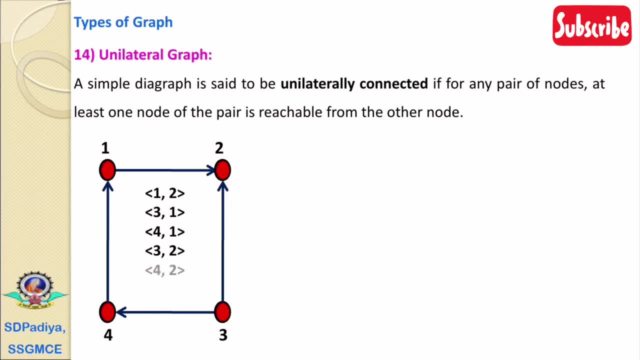 not has any outgoing age. Next, for a pair of 4 comma 2, we can reach at a 2 from the 4, that is, 4 to 1 and 1 to 2.. There is no any path from 2 to 2.. 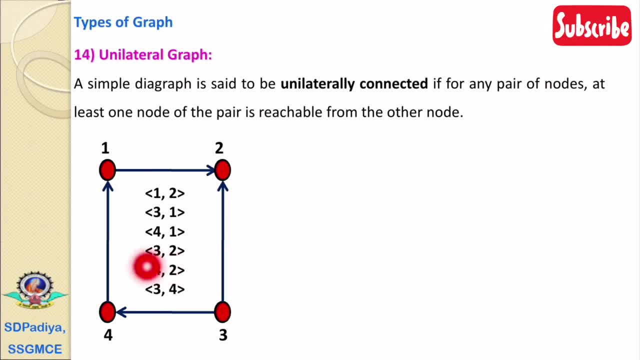 If you continue working in this direction then you will see, including a 3 comma. there is no any path from that side. For agai, there is no any path from 2 to 4.. For the last pair of 3imal 4 there is direct age, but there is no any path from 4 to 3.. 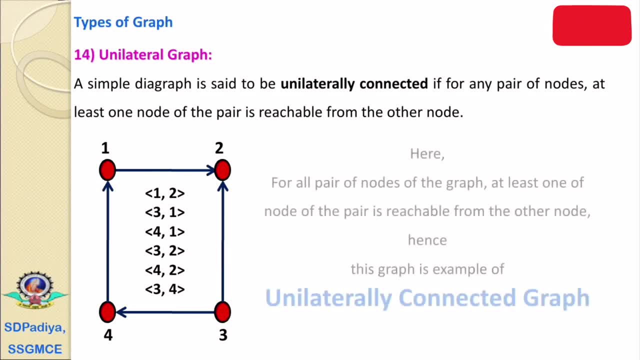 because we can move from 4 to 1 and one to 2. But there is no age from 2 to 3. Does not have in any 2 year pair of nodes of a graph. at least one of the node of the pair is reachable from the. 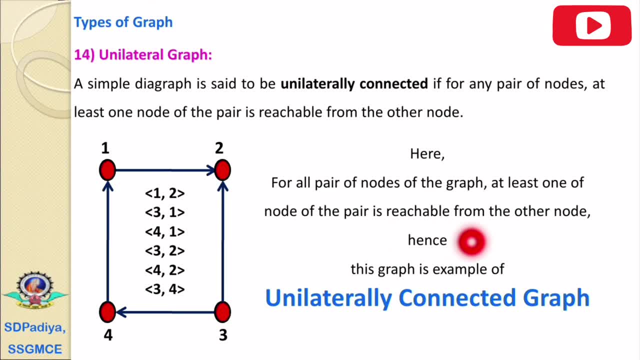 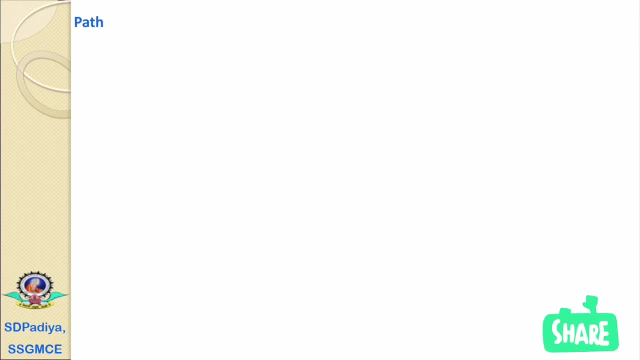 other node. Hence this graph is called the unilaterally connected graph. These are the types of the graphs. The next topic is about a path. There is a difference between the edge and path. The edge, it is a direct connection between any two nodes, and path it may be. 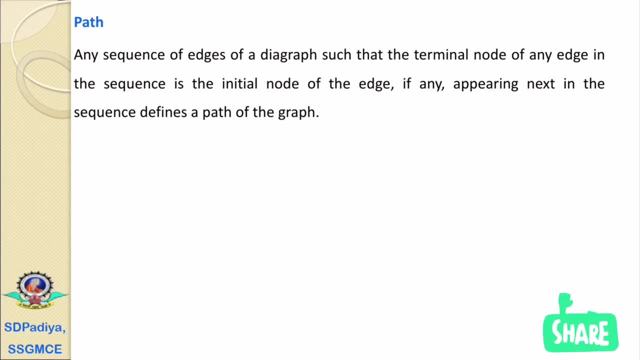 through any third node. Any sequence of edges of a diagram such that the terminal node of any edge in the sequence is the initial node of the edge, if any appearing next in the sequence defines a path of the graph. If we have the any three nodes, A, B, C. A is connected to the B and B is. 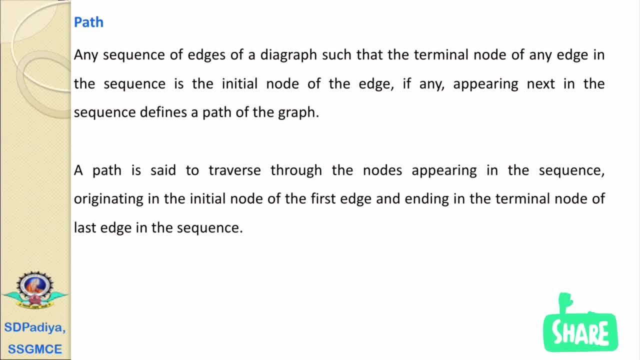 connected to the C. then we can say there is a path from A to C. A path is said to travels through the nodes appearing in the sequence, originating in the initial node of the first edge and ending in the terminal node of the last edge in the sequence: 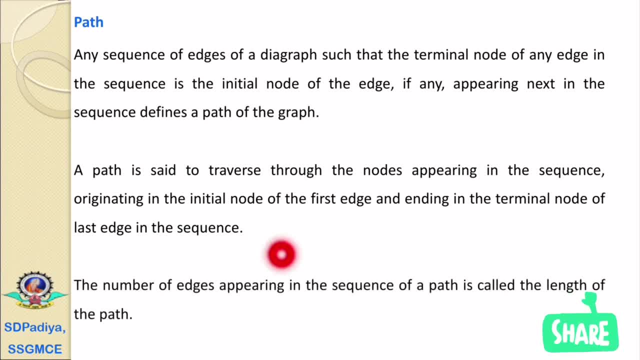 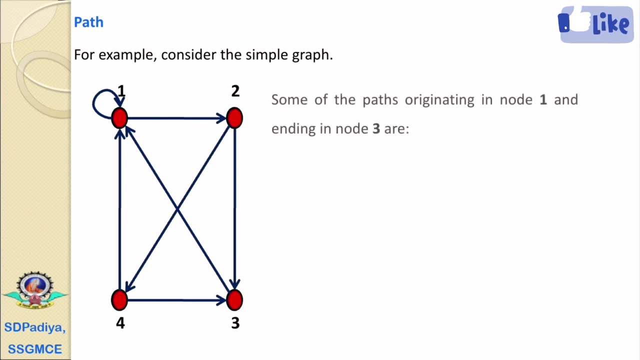 The number of edges appearing in the sequence of a path is called the length of the path. Let's have the example Example now. here suppose we have to find out the paths originating in the node 1 and ending in the node 3.. 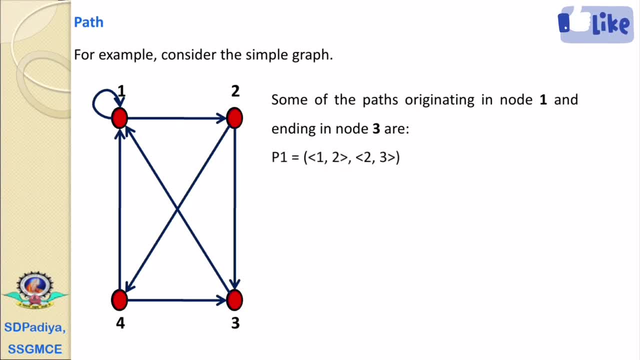 Then there are the different paths are available, which is originating at the node 1 and terminating at the node 3.. The first is edge 1, 2, 2 and 2, 2, 3.. There are the two edges. 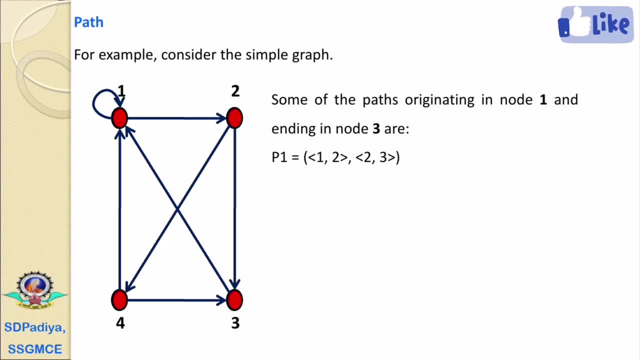 Therefore, the path length of the P1 is 2.. The second is an example from 1, 2, 2, 2, 2, 4 and 4, 2, 3 Z-like structure. There are the three edges in the path P2.. 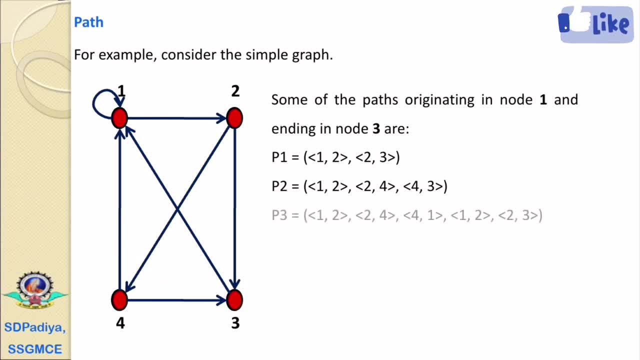 Hence its path length is 3.. Next is the 1,, 2,, 2,, 2,, 2,, 4,, 4,, 2,, 1.. Again 1,, 2,, 2, and then 2,, 2,, 3.. 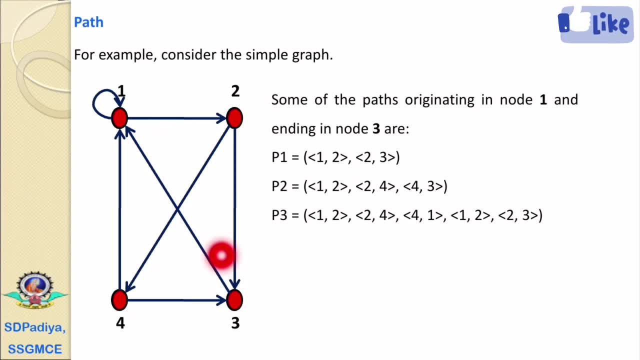 Next is the 1, 2, 2, 2, 2,, 4,, 4,, 2, 1.. In a path, the repetition of any edge and the vertex it is allowed. In this P3, there are 5 edges. 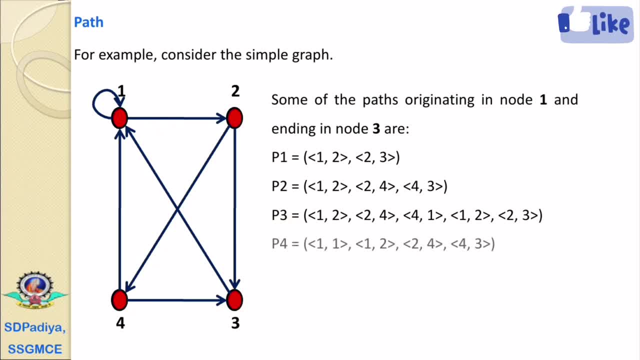 Hence its path length is 5.. Next is an example for P4.. The 1, 2, 1, because there is a loop, Then 1, 2, 2, 2, 2, 4 and 4, 2, 3.. 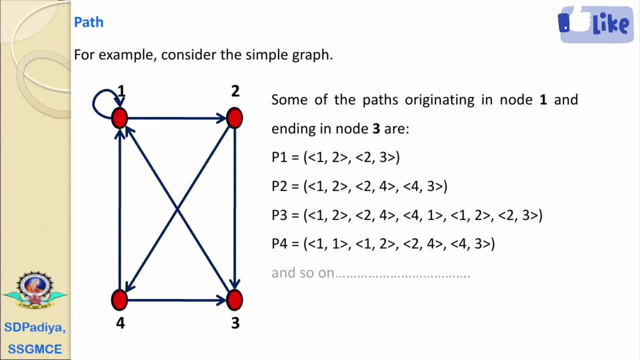 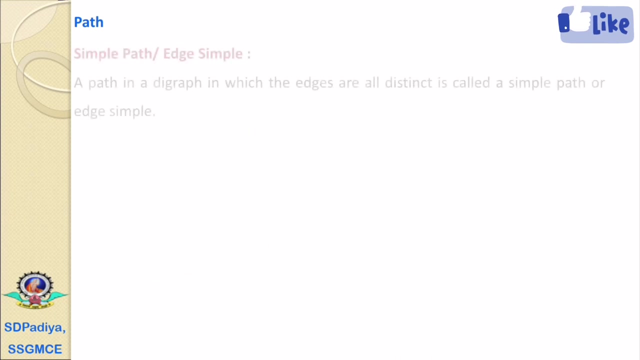 The path length for P4 is 4.. And so on. We can find out the path between the any two nodes which will travels through the any other node And the number of edges between any path. that is called a path length. There are the two types of the path. 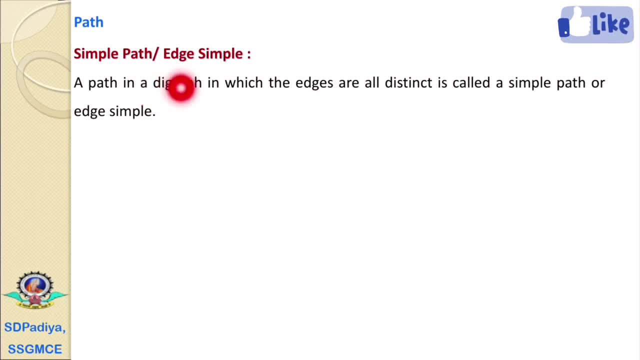 The first type is called a simple path or the edge. simple A path in a diagraph in which the edges are all distinct, all different, then it's called a simple path. or the edge. simple Means if in a path all the edges are different, no edge is repeated, then it is called a simple path. 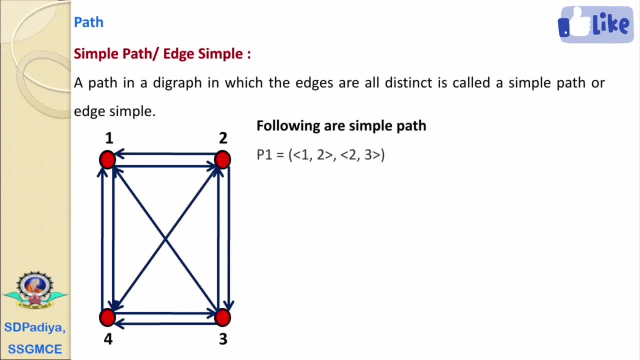 Let's have an example: The path 1, 2, 2 and 2,, 2, 3,. there is no any repetition. all these two edges are different. therefore P1, it is a simple path. 1, 2, 4 and 4,, 2, 3, again, there is no any repetition, it is a simple path. 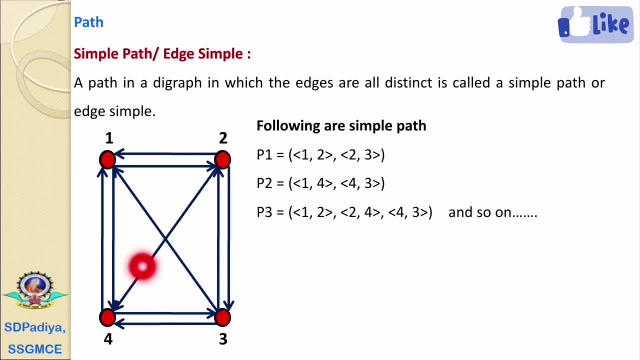 The P3 is the 1, 2, 2, 2, 2, 4 and 4, 2, 3, z-like structure. Again, there is no any repetition of the edge. all the edges are distinct. 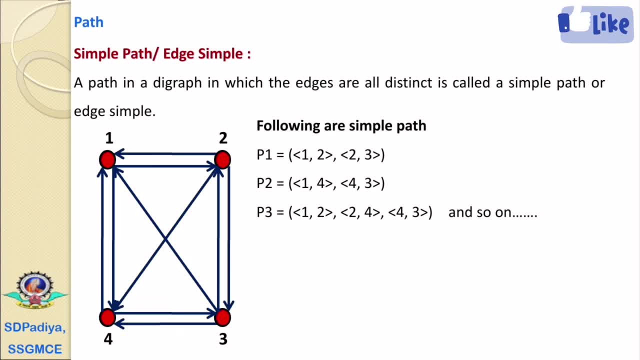 Hence it is a simple path, and so on. Now we will discuss that which are not the simple path. Suppose we consider a path from 1, 2, 2 to 2, 3,, then 3, 2, 1,, again 1, 2, 2 and 2, 2, 3.. 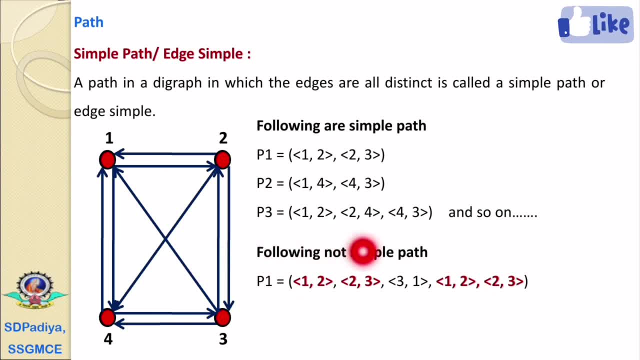 Now, in this the two edges are repeating, that is, 1, 2, 2 and 2, 2, 3.. Hence it is not considered as a simple path. The next is a example. Suppose we have a path from 1, 2, 4, 4, 2, 3, 3, 2, 1,, again 1, 2, 4 and 4, 2, 3.. 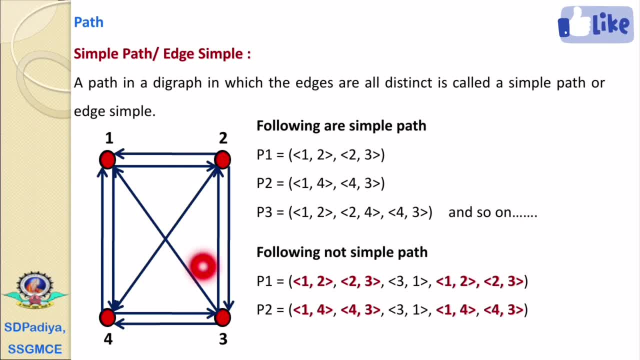 Then again there are the repetition of the two edges, therefore not considered as a simple path. The P3 is the 2, 2, 3, it is starting from the node 2, 2, 2, 3, 3, 2, 4.. 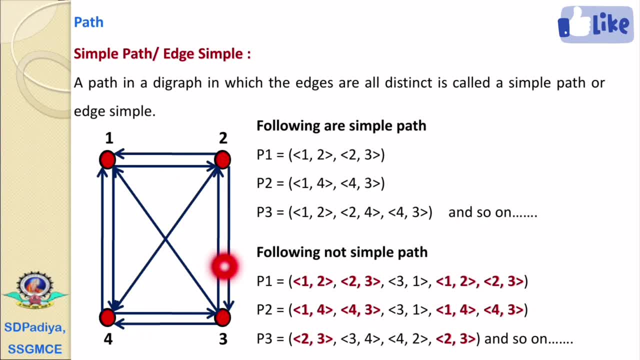 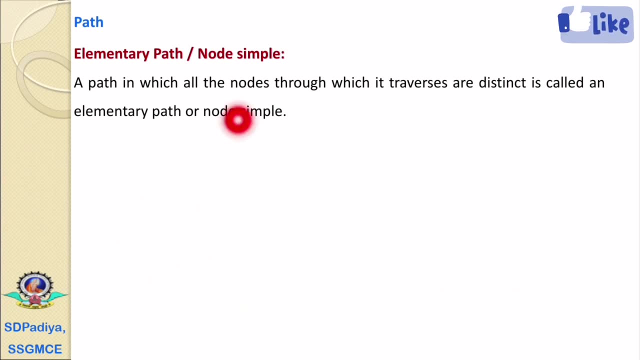 4,, 2,, 2.. And again 2,, 2,, 3, a triangle. then in that a node, 2,, 2,, 3 is repeated, therefore not considered as a simple path, and so on. The second type is elementary path, or called a node simple. 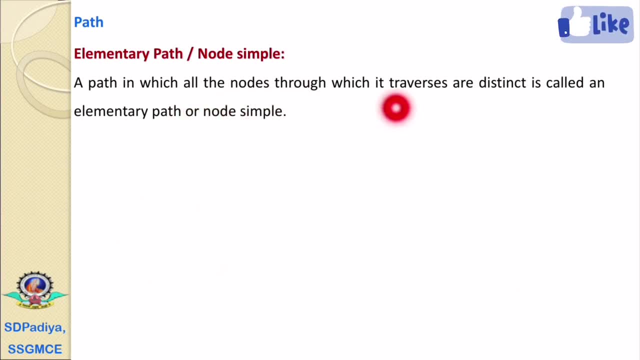 A path in which all the nodes through which it is traverses are distinct Means. if in a path no node is repeated, then it is called An elementary path or the node, simple, Again with the same graph. we will discuss the some paths for the elementary path. 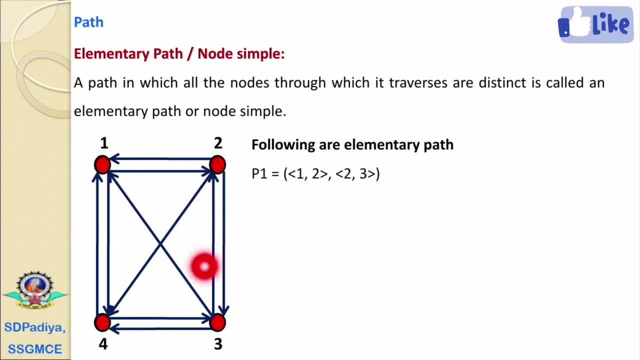 The first is the 1, 2, 2 and 2, 2, 3.. There is no any repetition of the node, Hence it is the elementary path. Second is a path from 1, 2, 4 and 4, 2, 3.. 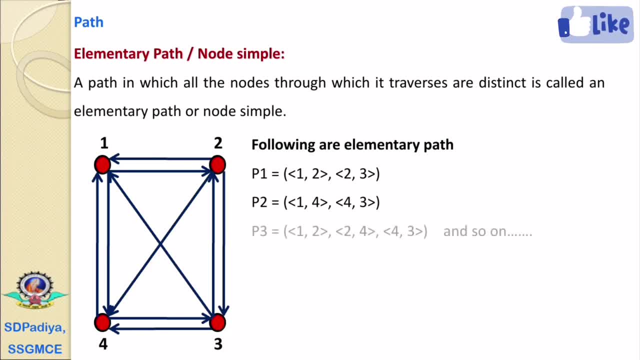 There is again no repetition. then it is considered as elementary path. The next is a path from 1, 2, 2.. 2, 2, 4 and 4, 2, 3.. The Z-like structure. 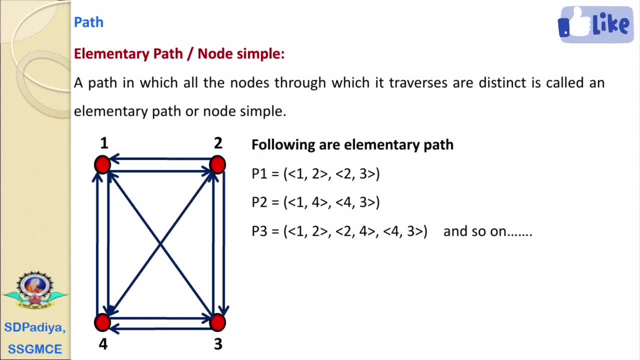 Again, no node is repeated, hence considered as an elementary path. Now we will discuss which are not the elementary path. Suppose we have a path that is 1, 2, 2, 2, 2, 3, then 3, 2, 1.. 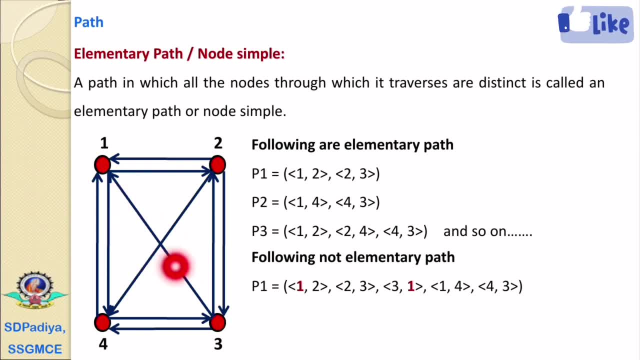 1, 2, 4 and then 4, 2, 3.. Now, in this No edge is repeated, but the node 1, it is repeated because we have already started from the one, that is, 1, 2, 2, 2, 2, 3, and then 3, 2, 1, and 1, 2, 4, the node 1, it is repeated, hence it is not considered as an elementary path, but it is an example for simple path, because edge is not repeated. 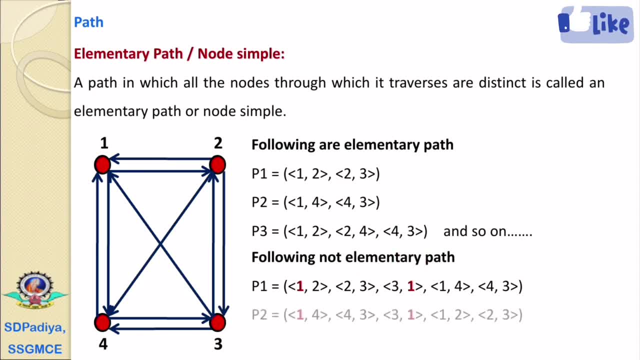 Every edge is a unique. The second is an example: The 1,, 2,, 4,, 4,, 2,, 3,, 3,, 2,, 1,, 1,, 2,, 2,, and then from 2 to 3.. 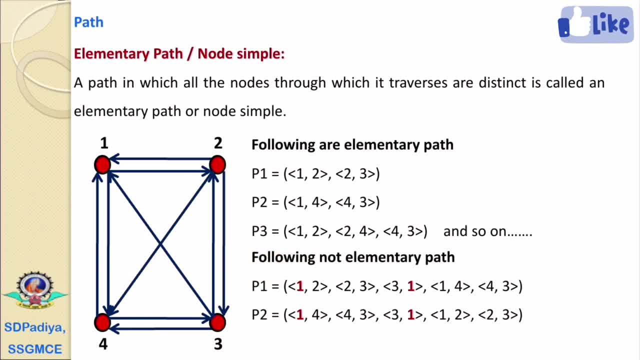 Again, in that the node 1, it is repeating. It is repeating node, hence it is not an elementary path. But if we look in this P2,, again there is no any repeated edge. hence it is an example for simple path. 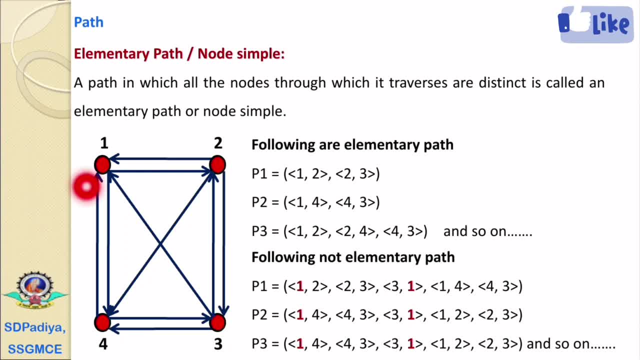 The third is P3, the 1,, 2,, 4,, 4,, 2,, 3,, 3, 2, 1, 1,, 2,, 2, and 2,, 2, 3, similar as above. we have example and so on. 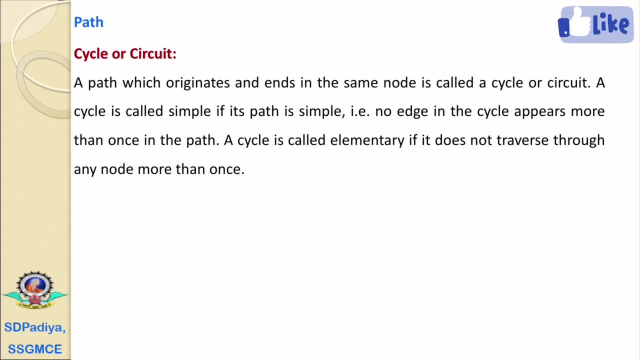 The next type of the path is cycle or circuit. A path which originates and ends in the same node is called a cycle or circuit. A cycle is called simple If its path is simple. that is no edge in the cycle. appears more than 1 in the path. 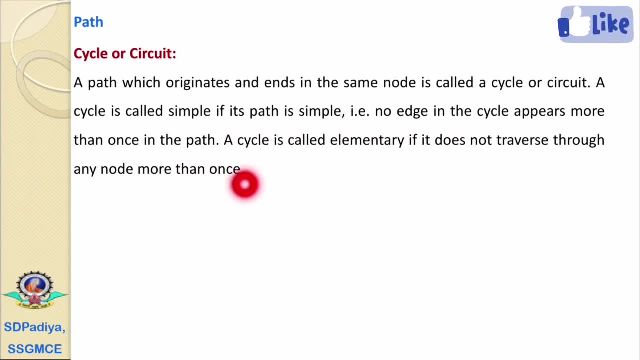 And a cycle is called elementary if it does not travels through any node more than 1.. Means again, there are the two types of the cycle. First, simple cycle, and second is an elementary cycle. If in a cycle every edge is a unique, then it is called simple cycle. 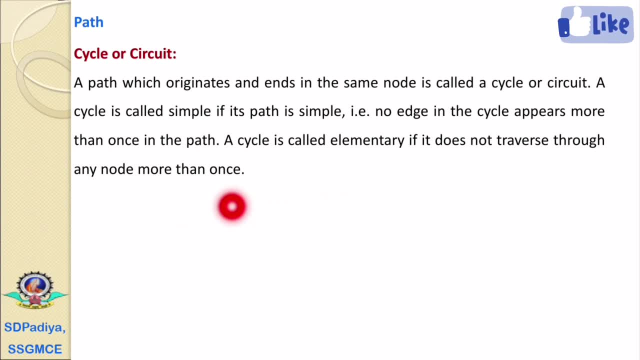 And if in a cycle every node is unique, then it is called elementary cycle. Lets have the example. The following are the cyclic path, The P1, that is, 1, 2, 2, 2, 2, 3, and 3, 2, 1, the triangle. 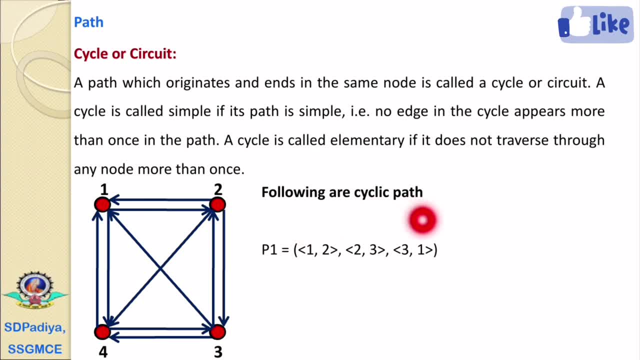 Means we are starting at a 1 and we are ending at a 1.. Now, in this, every edge is a unique and every node is a unique. There is no repetition. Hence the P1. it is a simple cycle. The second P2, 1, 2, 4, 4, 2, 3, and 3, 2, 1,. again, in this, every edge is a unique and every node is a unique. 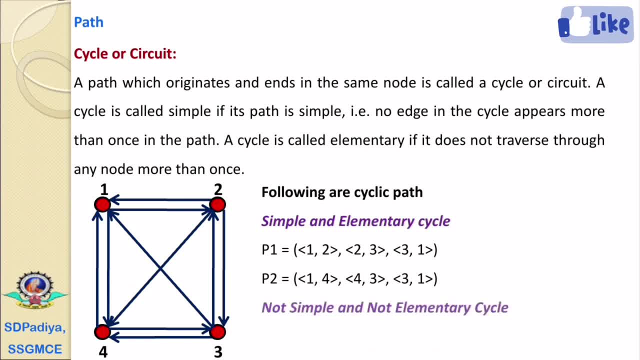 No repetition. therefore. it is also the example for simple cyclic path and elementary cyclic path. Now, at last, we will discuss which is a path, not a simple path. Now, at last, we will discuss which is a path, not a simple path. It is a simple and not elementary cycle. 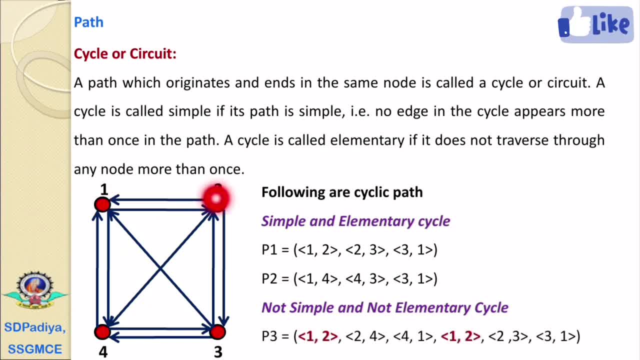 Lets have a cyclic path that is, 1, 2,, 2,, 2,, 2,, 4,, 4, 1.. Then 1, 2, 2,, 2,, 2, 3, and at last, 3, 2, 1.. 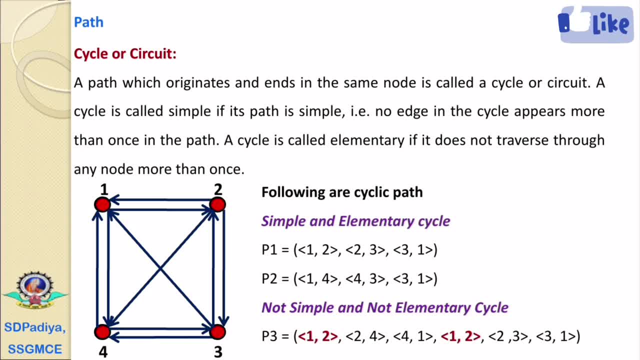 This path is starting at 1 and ending at 1.. Therefore, it is a cyclic, But the edge 1, 2,, 2, it is repeated, It is two times use And the node 1 and node 2..